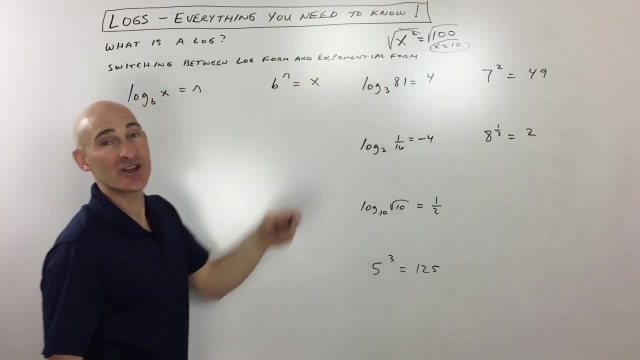 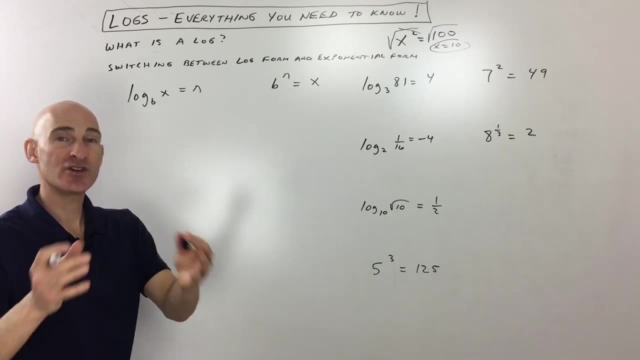 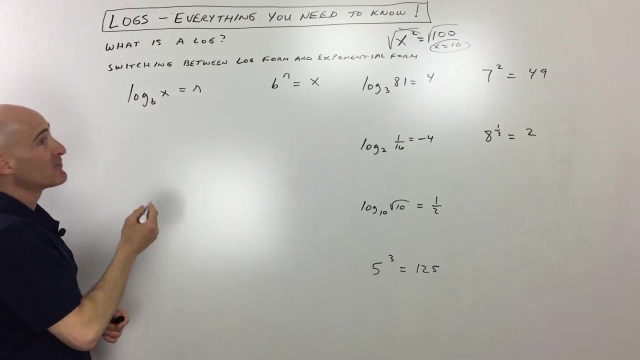 unfamiliar to us right now, to the more familiar exponential form, And I'm going to show you a way to do that. So, as logs and exponential functions are inverses, what we can do is we can use that to our advantage. So, if we've got log, base b of x equals n, what I can do is I can. 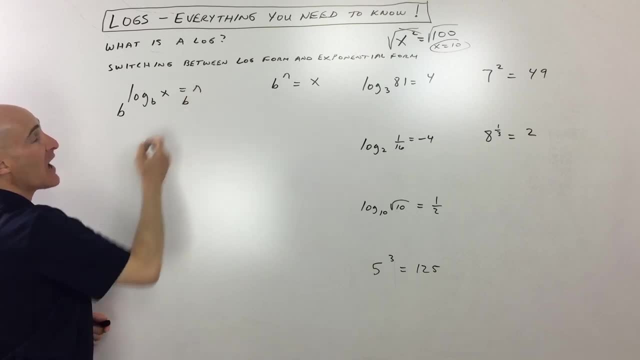 exponentiate both sides okay, of this equation using the same base, as long as these bases match. So those are going to cancel each other out. And now we have x equals b to the n right. So now it's in our exponential form. We're going to go through some examples so you can see how this. 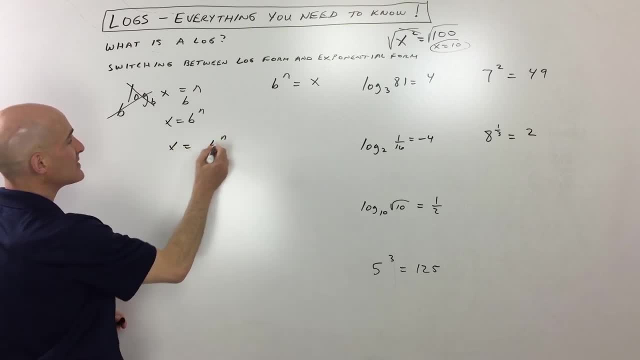 works. Now, if it was in this form, x equals b to the n right. So now it's in our exponential form: b to the n. see, this is the base, This is the exponent. What I'm going to do is I'm going to 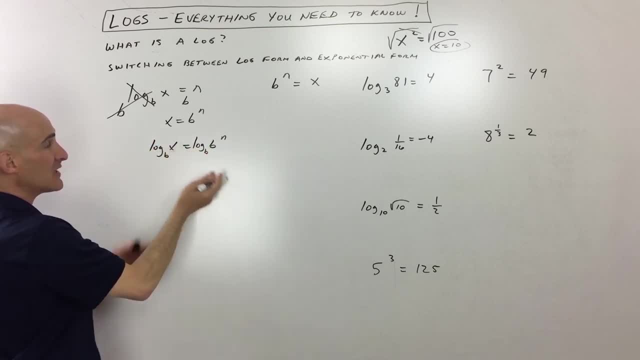 take the log base b of both sides. okay, to keep it balanced. Remember, in algebra you want to do the same thing to the left and the right sides, But the log base b and the exponential function with base b, those cancel one another out. And now you can see we're back to where we started. 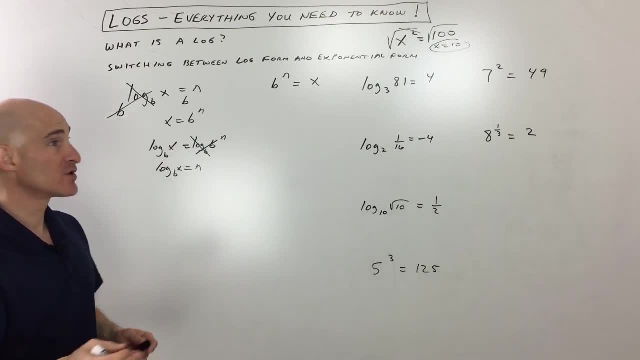 originally. So understanding how to switch between the two forms is really key. Now a lot of teachers, okay, will teach their students this And they'll say: this is the base. okay, This number here. it's like a subscript. It's a little bit below the. 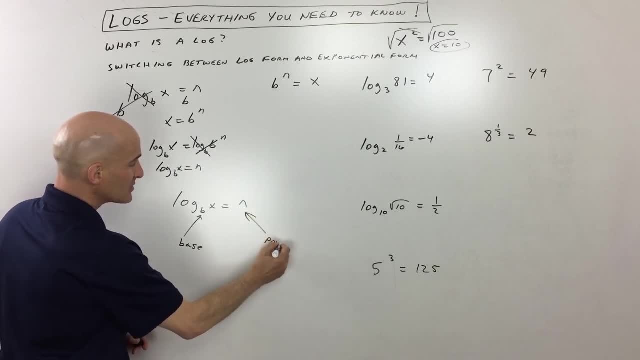 line, this b And this is the power. okay, So n is the power, That's your exponent, And then the x, that's your answer, or oftentimes referred to as the argument. okay, Not like getting into a fight. 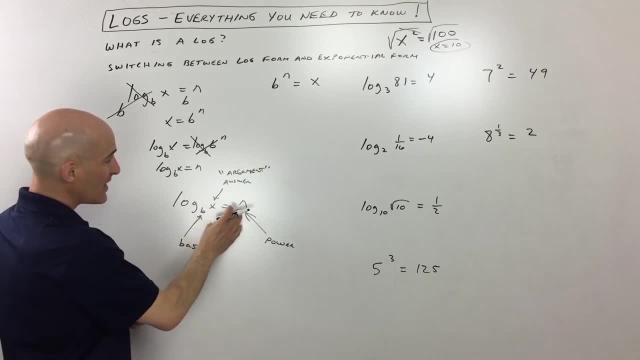 okay, Just the argument, That's the answer. So if you know that's the base, that's the power, that's the answer, then you can say: okay, there's my base, there's my power, there's my answer. 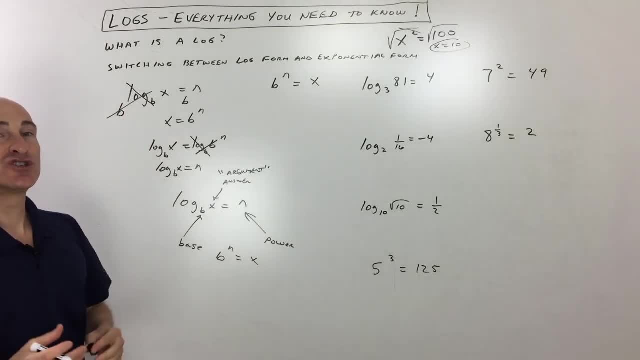 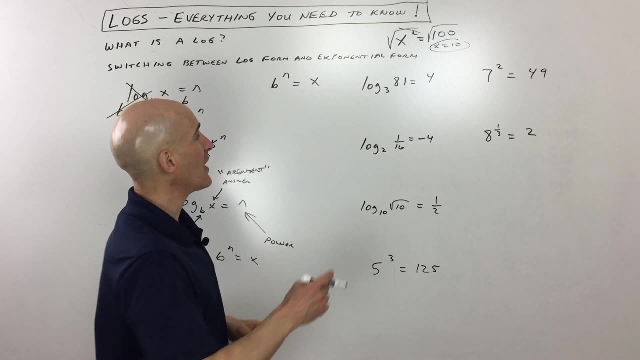 okay, I'm going to show you this Because I think it's a little bit more intuitive and easy to understand. So let's go through a bunch of examples here. So let's switch this from the log form to the exponential form. We'll do. 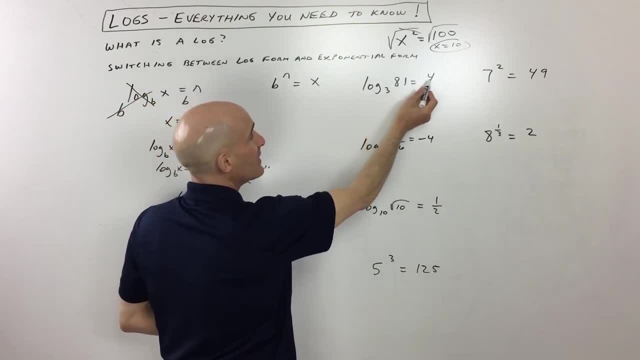 that first. So you've got log base three of 81 equals four. So what I'm going to do is I'm going to exponentiate both sides, I'm going to raise both sides using the base three. Why? Because exponential functions and logarithmic functions. they're inverses, just like we talked about. 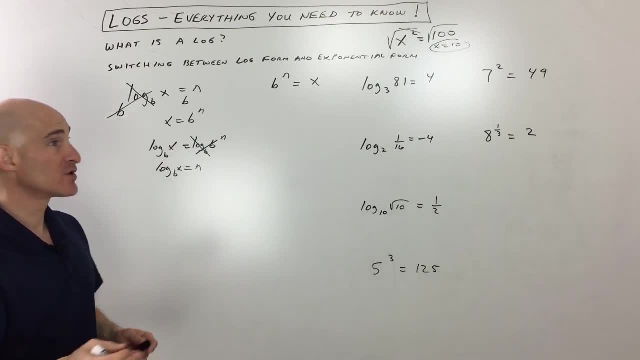 originally. So understanding how to switch between the two forms is really key. Now a lot of teachers, okay, will teach their students this And they'll say: this is the base. okay, This number here. it's like a subscript. It's a little bit below the. 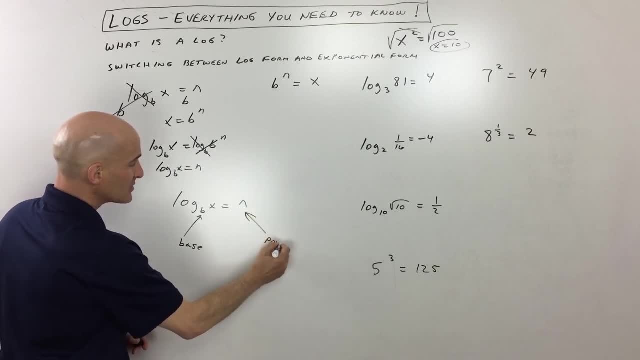 line, this b And this is the power. okay, So n is the power, That's your exponent, And then the x, that's your answer, or oftentimes referred to as the argument. okay, Not like getting into a fight. 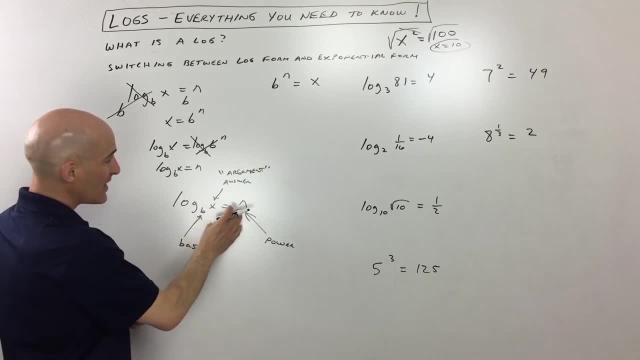 okay, Just the argument, That's the answer. So if you know that's the base, that's the power, that's the answer, then you can say: okay, there's my base, there's my power, there's my answer. 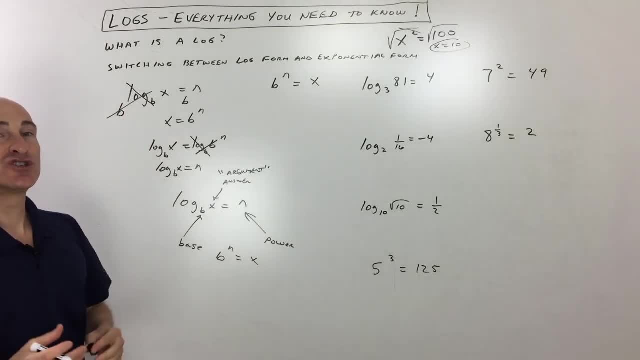 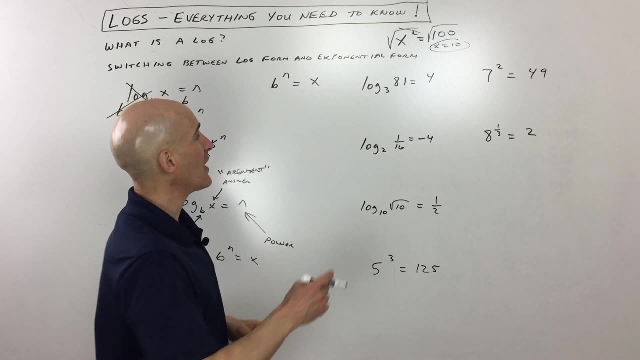 okay, I'm going to show you this Because I think it's a little bit more intuitive and easy to understand. So let's go through a bunch of examples here. So let's switch this from the log form to the exponential form. We'll do. 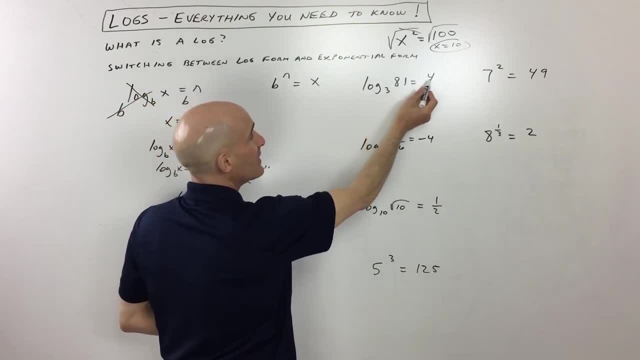 that first. So you've got log base three of 81 equals four. So what I'm going to do is I'm going to exponentiate both sides, I'm going to raise both sides using the base three. Why? Because exponential functions and logarithmic functions. they're inverses, just like we talked about. 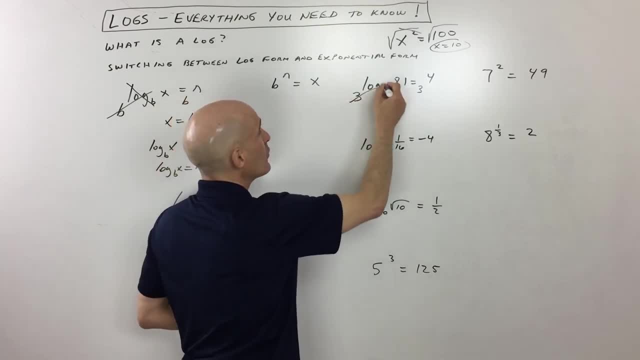 earlier, squaring and square rooting, multiplying, dividing, adding, subtracting. When you do that, they cancel one another out. Okay, So now you've got three to the fourth, power equals 81, which we know is true Three times three. 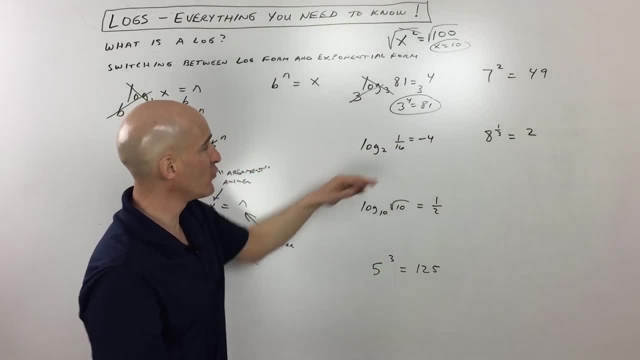 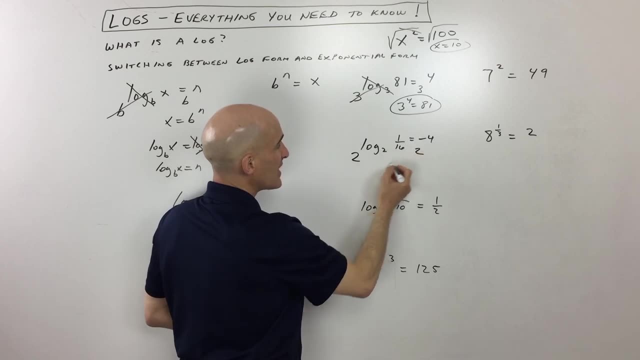 times three times three is 81. Okay, How about this? one Log base two of 1: 16th. Well, again, we're going to exponentiate using the same base, Log base two. exponentiate both sides using base two. Those are inverses, They cancel. So now you can see we've got two to the negative, four equals. 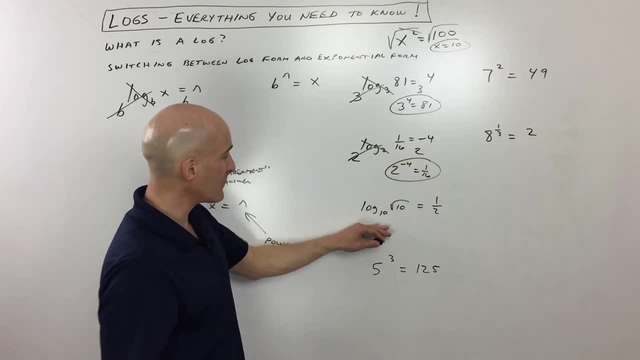 1, 16th and you've got it. Let's go down to this one log, base 10.. So now, what I'm going to do is I'm going to exponentiate both sides using the base 3.. Now you're going to be able to do that. 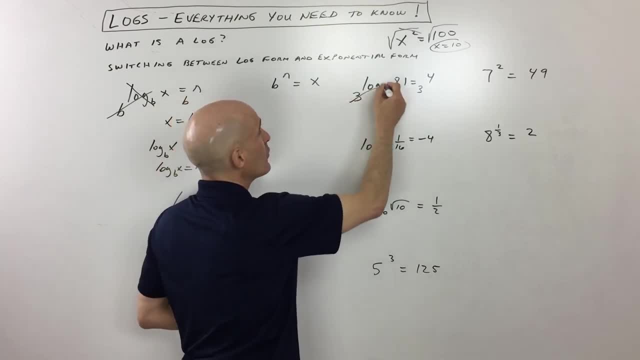 earlier, squaring and square rooting, multiplying, dividing, adding, subtracting. When you do that, they cancel one another out. Okay, So now you've got three to the fourth, power equals 81, which we know is true Three times. 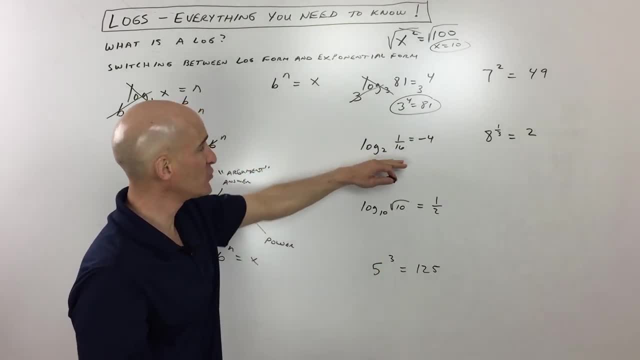 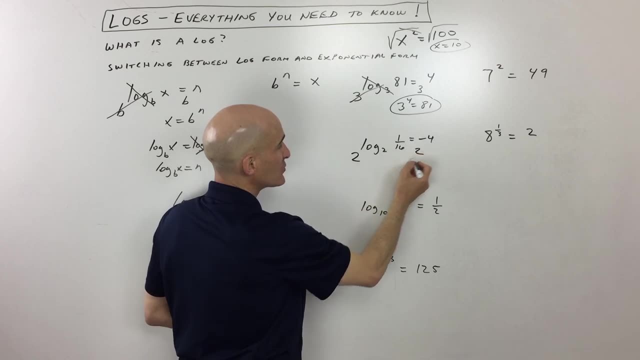 three times. three times three is 81. Okay, How about this? one log base two of one. sixteenth. Well, again, we're going to exponentiate using the same base, log base two. exponentiate both sides using base two. Those are inverses, They cancel. So now you can see. 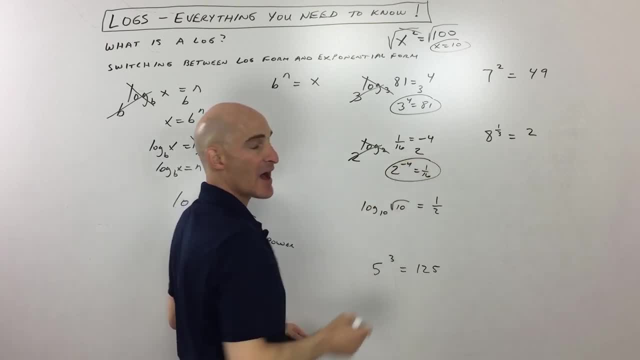 we've got two to the negative. four equals one, sixteenth, and you've got it. Let's go down to this one log, base 10.. So now what I'm going to do is I'm going to exponentiate both sides using base 10. those undo one another, and we've got 10 to the 1. half power equals the. 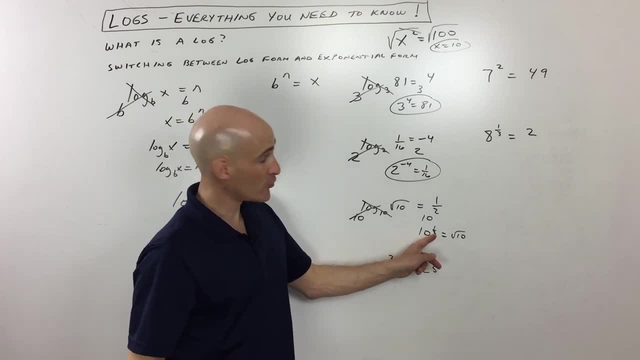 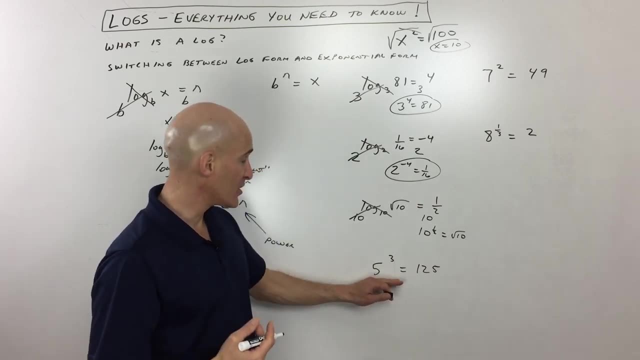 square root of 10, and remember your fractional exponents. the denominator is the root, so that's why that's the square root of 10. this is 10 to the first power. now we're gonna go the other direction. okay, we're gonna switch from the. 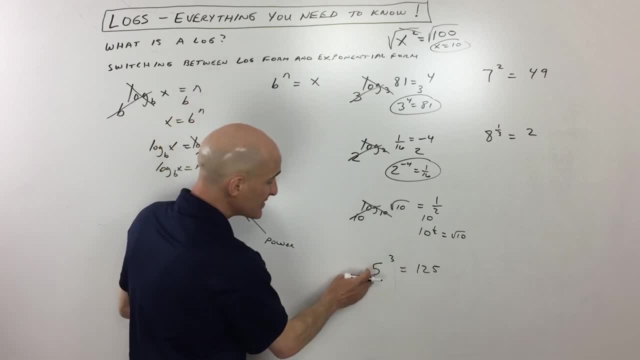 exponential form to the logarithmic form. this is the base log. okay, so this is base 5. so we're gonna take the log base 5 of both sides. these are inverses, they cancel. so we get 3 equals log base 5 of 125. now you can write it either way, but 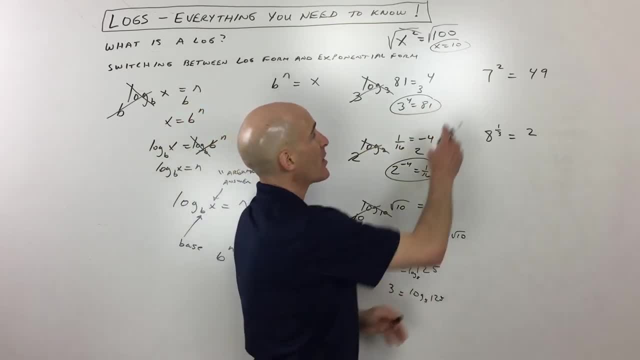 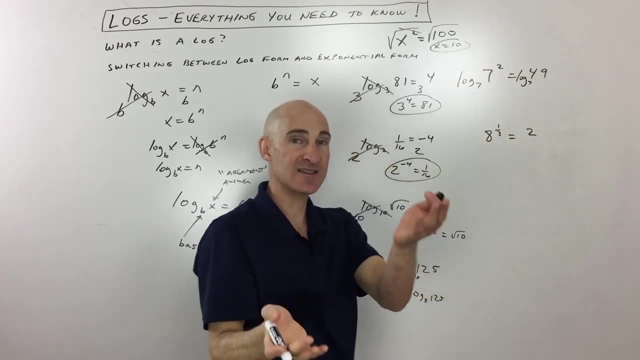 I'm just gonna leave that like that for right now this one. we've got 7 squared. 7 is the base, so let's go ahead and do the inverse of exponentiating with base 7. let's take the log base 7 of both sides to keep it balanced. these are: 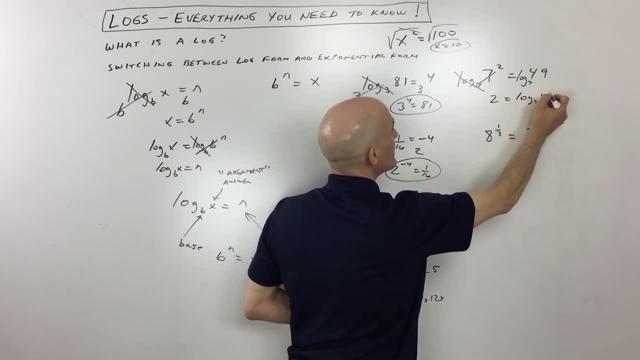 inverses. they undo one another. so you can see: log base 7 of 49 equals 2 and you got it last one here for this group of problems. we're gonna take the log base 8 of both sides. those are inverses and now you've got 1. 3rd equals log base 8 of 2. now, if you 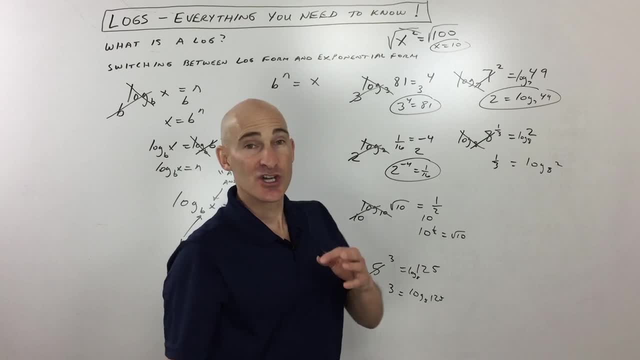 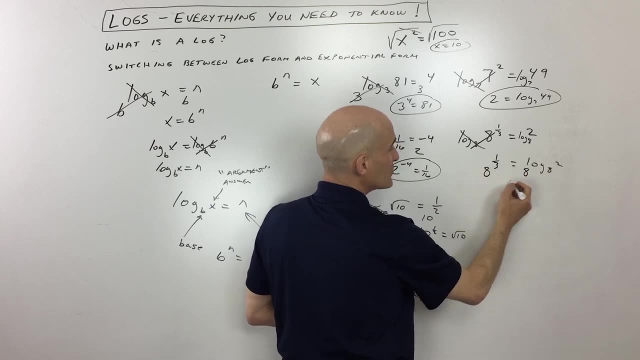 want to get more comfortable with this process, just keep switching back and forth between the two forms. and what I mean by that is see how you have log base 8. let's just exponentiate both sides using base 8. those are inverses. now we get back what we had at the very beginning. let's say we want to take the. 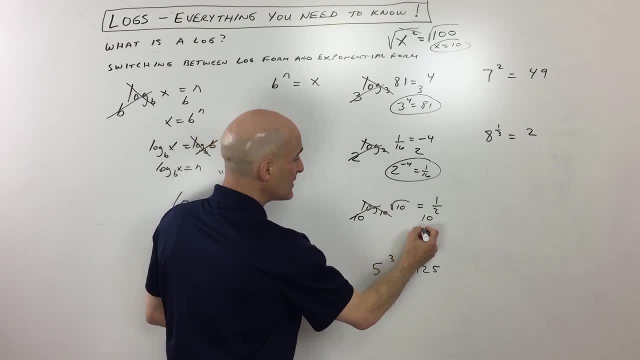 So you're going to go down to this one log, base 10.. So now what I'm going to do is I'm going to Using base 10, those undo one another and we've got 10 to the 1 1⁄2 power. 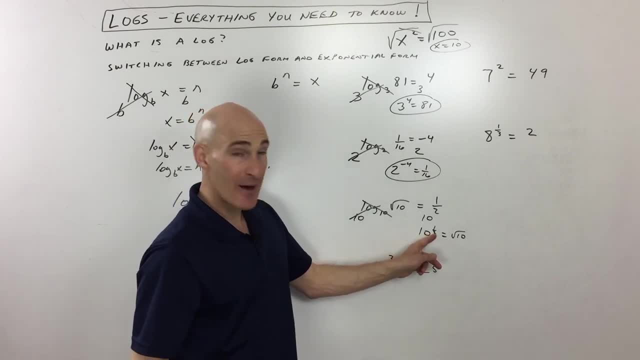 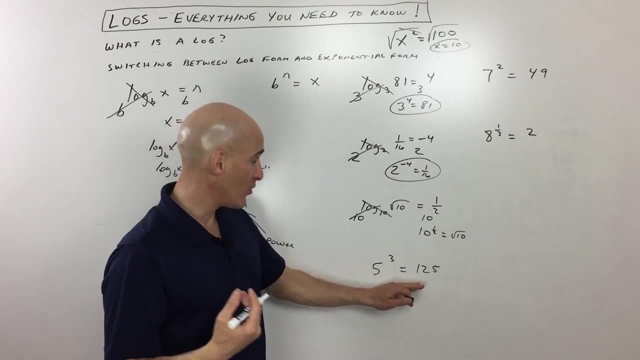 equals the square root of 10.. And remember your fractional exponents. the denominator is the root, so that's why that's the square root of 10.. This is 10 to the 1st power. Now we're gonna go the other direction. 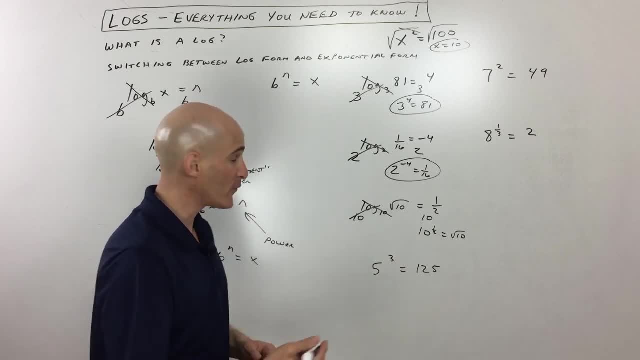 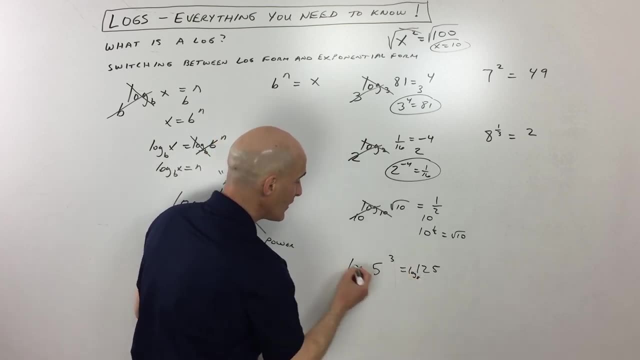 Okay, we're gonna switch from the exponential form to the logarithmic form. This is the base log. okay, so this is base five. so we're gonna take the log base five of both sides. These are inverses. they cancel. 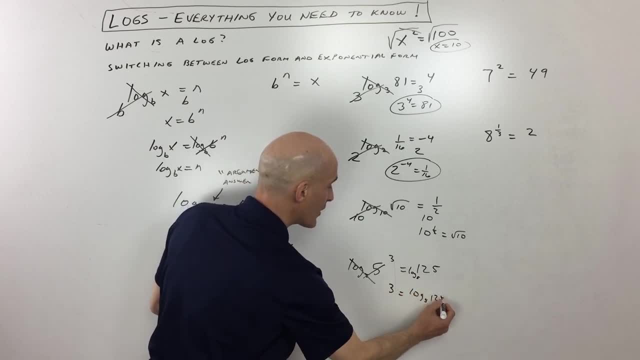 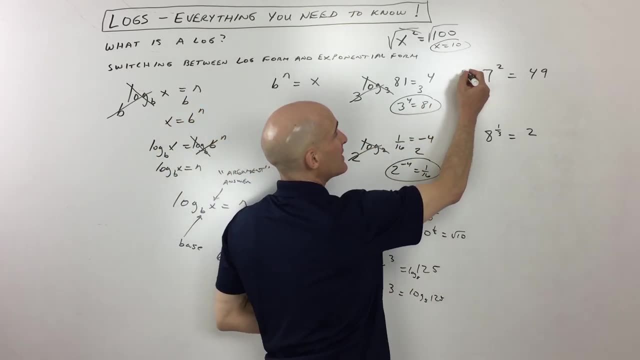 so we get three equals log base, five of 125.. Now you can write it either way, but I'm just gonna leave it like that for right now. This one. we've got seven squared. seven is the base, so let's go ahead and do the inverse. 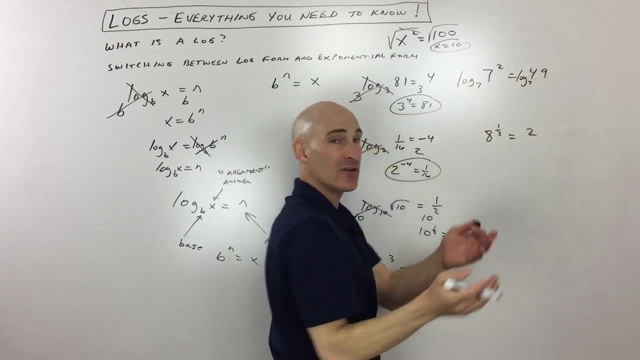 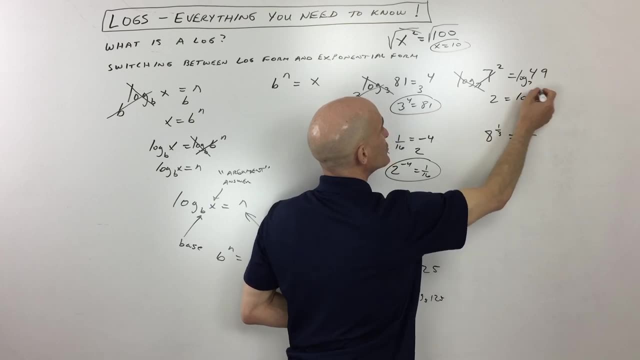 of exponentiating with base seven. Let's take the log base seven of both sides. to keep it balanced, These are inverses, they undo one another. so you can see: log base seven of 49 equals two. and you got it. Last one here for this group of problems. 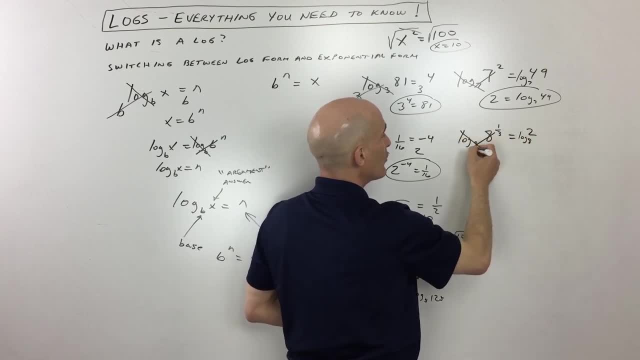 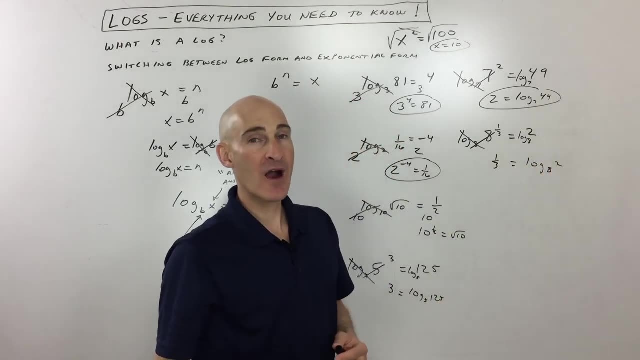 we're gonna take the log base eight of both sides. those are inverses. and now you've got one third equals log base eight of two. Now if you wanna get more comfortable with this process, just keep switching back and forth between the two forms. 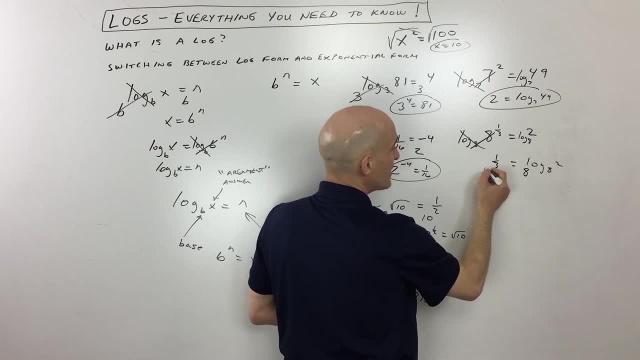 and what I mean by that is see how you have log base eight. Let's just exponentiate both sides using base eight. Those are inverses. Now we get back what we had at the very beginning. Let's say we wanna take the log base eight again. 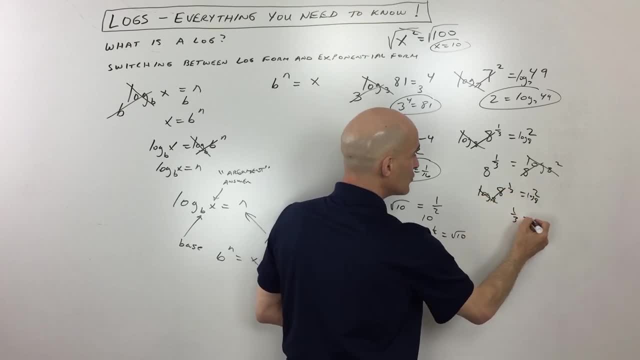 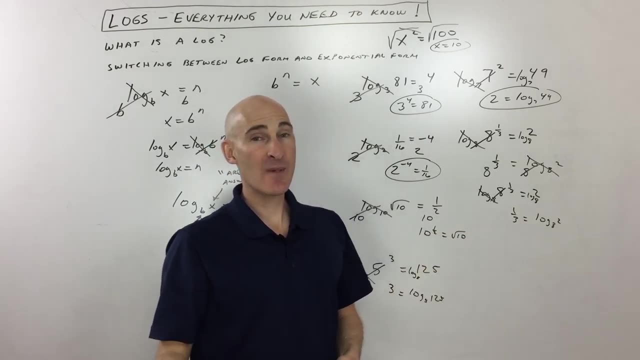 on both sides. right, Those are inverses and we're back to the logarithmic form, and you can keep doing that forever and ever until you feel really comfortable with switching the forms. So that's my preferred method, just because I feel like it's more intuitive. 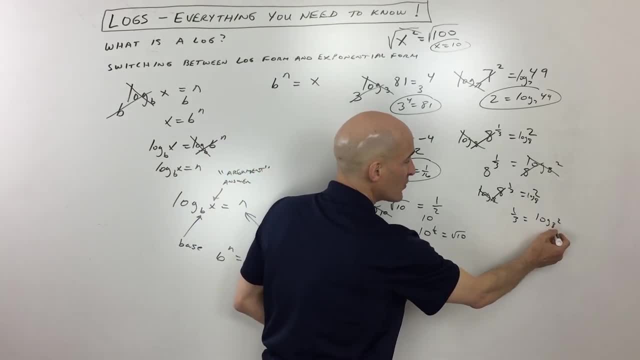 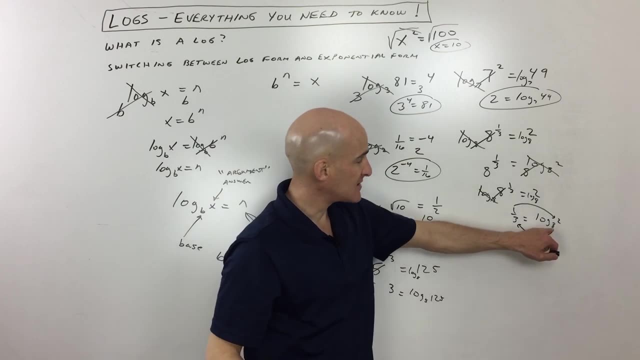 but if you don't like that method, stick with what you like. Some teachers will even just use this circle technique. They'll say: this base raised to this power equals that answer. But just remember, that's the base, that's the power of the exponent. 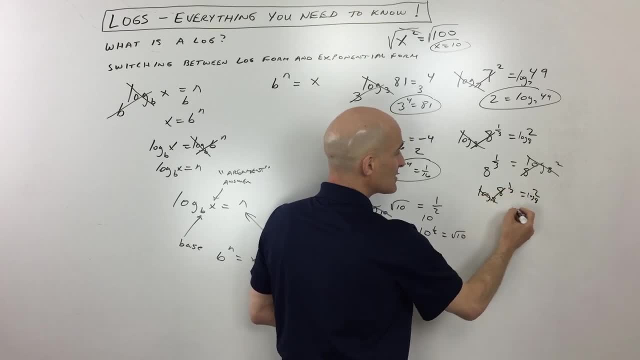 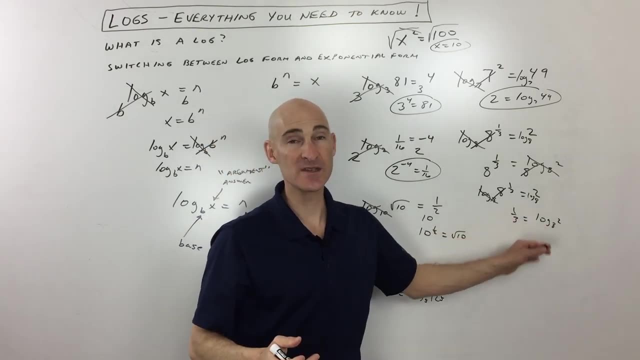 log base 8, again on both sides right, those are inverses and we're back to the logarithmic form and you can keep doing that for a forever and ever until you feel really comfortable with switching the forms. so that's my preferred method, just because I feel like it's more intuitive. but if 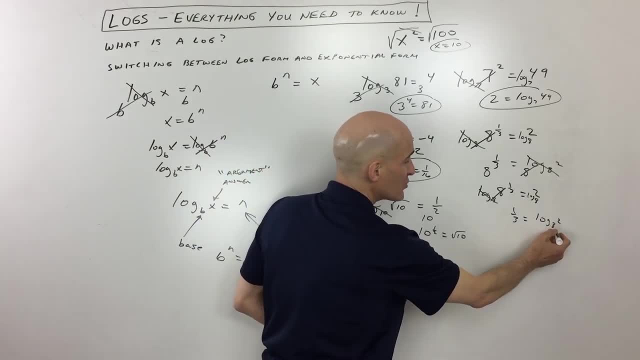 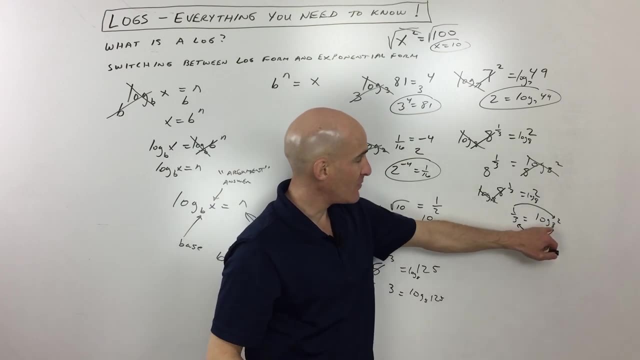 you don't like that method, stick with what you like. some teachers will even just use this circle technique. they'll say: this base raised to this power equals that answer. but just remember that's the base, that's the power of the exponent, and then the 2- the argument, is the answer. so the next step in logarithms: 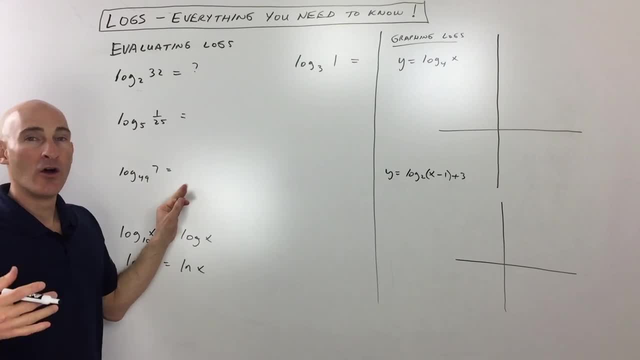 we're going to get into. let me erase this board and we'll get right back at you. okay, now we're going to talk about evaluating logs. so when they say evaluate, what does that mean? it just means find the value. in the last part that we were talking about, we were switching forms between the 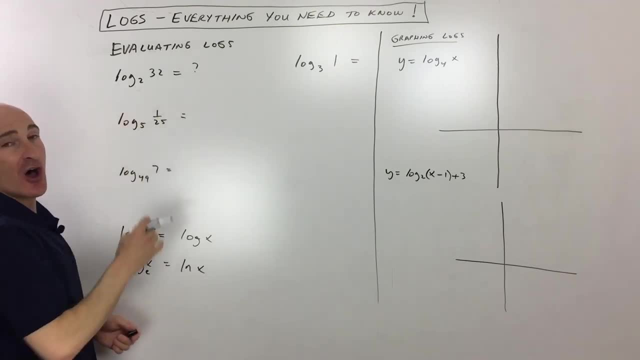 exponential and logarithmic forms. but now what we're doing is we're actually solving, we're actually getting an answer, and what you can do is you can do the same thing, like we were doing in the last part: just go ahead and exponentiate both sides of the equation, so the exponential function, the logarithmic, 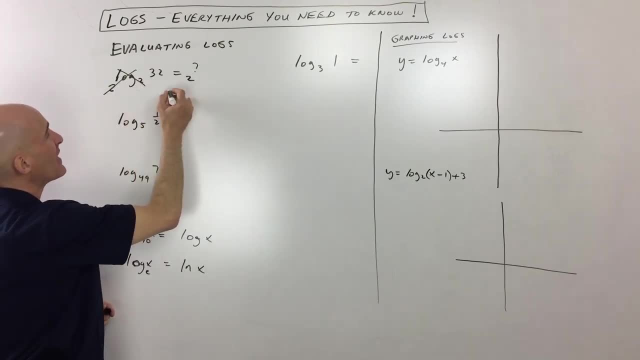 function. they cancel one another out as long as the bases are the same. so now what we have is: 2 to what power equals 32. well, you can see that's going to be 5. now, oftentimes what I recommend to students is just put a variable here, like X, for example. so log base: 5 of 125. 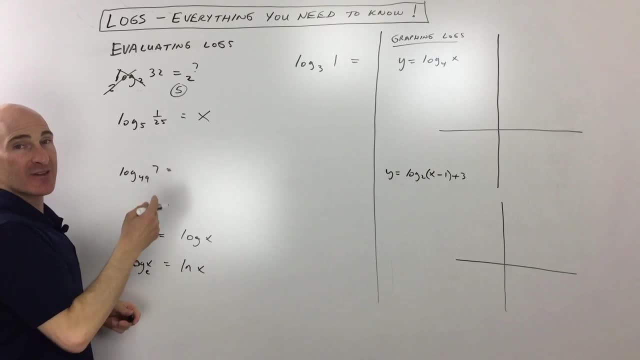 equals X, right? so we're not as familiar of thinking in terms of logs, so let's go ahead and exponentiate both sides. make sure that these bases are the same. they're inverses, they cancel each other out. 5 to what power is 125th negative 2? 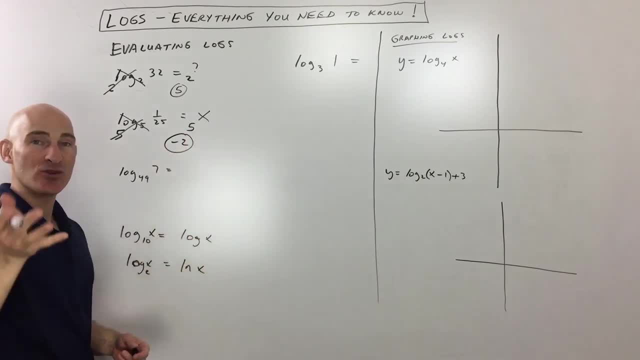 because 5 squared is 25, but the negative exponent takes the reciprocal right. this one here log base 49 of 7. again, we're just going to make it equal to a variable x. we're going to exponentiate both sides, right? so those are inverses: 49 to what power is 7? 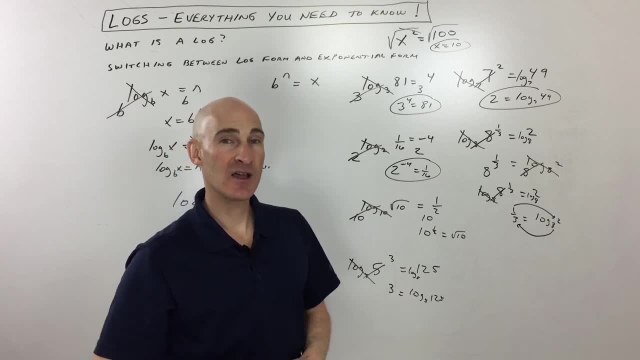 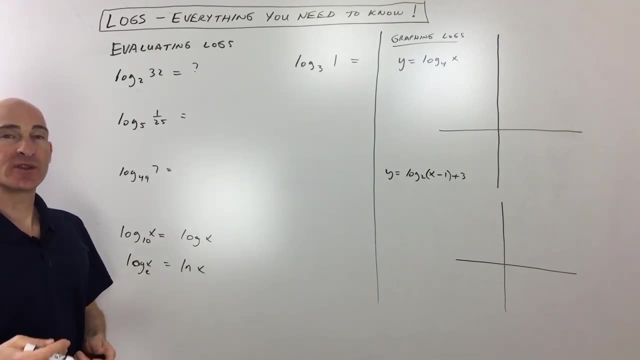 and then the two of the argument is the answer. So the next step in logarithms we're gonna get into, let me erase this board and we'll get right back at you. Okay, now we're gonna talk about evaluating logs. So when they say evaluate, what does that mean? 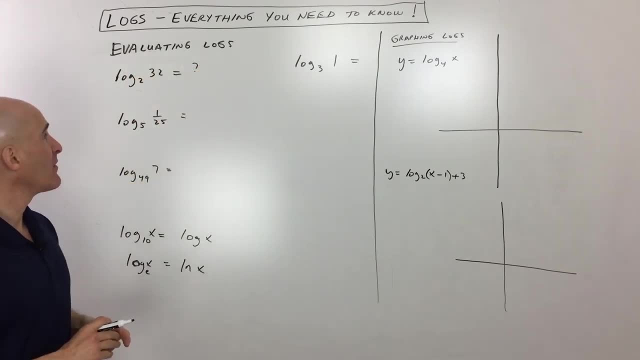 It just means find the value. In the last part that we were talking about, we were switching forms between the exponential and logarithmic forms. But now what we're doing is we're actually solving, we're actually getting an answer, And what you can do is you can do the same thing. 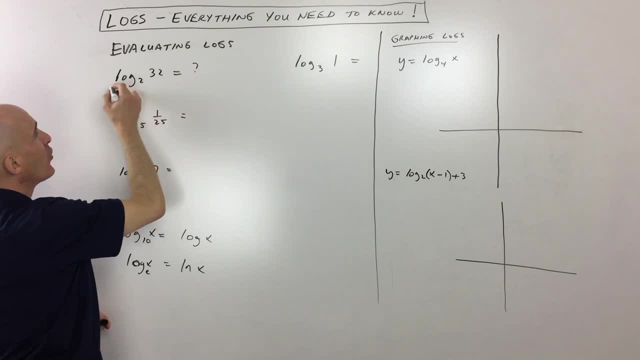 like we were doing in the last part, just go ahead and exponentiate both sides of the equation, So the exponential function, the logarithmic function, they cancel one another out as long as the bases are the same. So now what we have is two to what power? 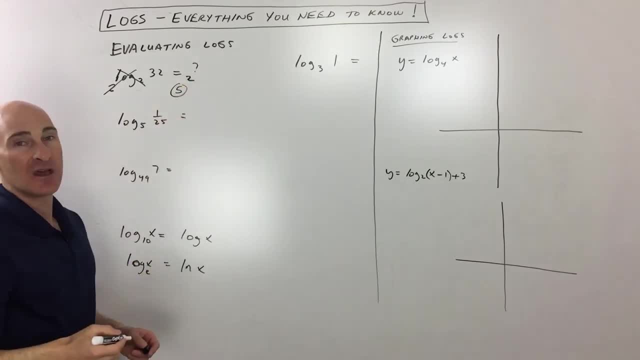 Equals 32.. Well, you can see that's gonna be five. Now, oftentimes what I recommend to students is just put a variable here, like x, for example. So log base five of 1- 25th equals x, right? So we're not as familiar of thinking in terms of logs. 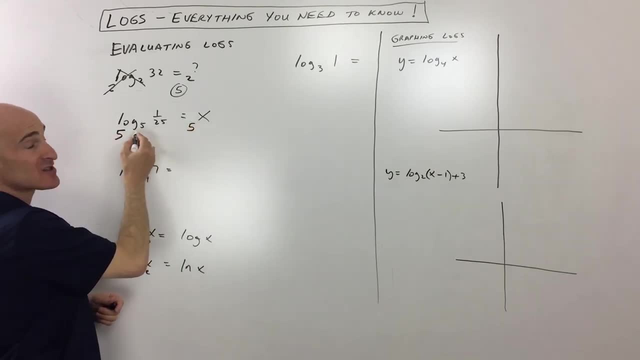 so let's go ahead and exponentiate both sides. Make sure that these bases are the same. They're inverses, they cancel each other out. Five to what power is 1? 25th Negative two, because five squared is 25,. 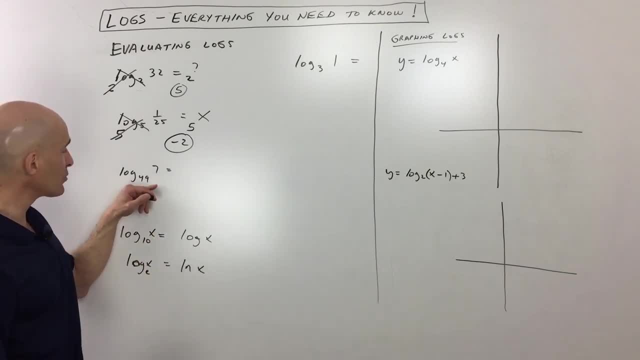 but the negative exponent takes the reciprocal right. This one here, log base 49 of seven. Again, we're just gonna make it equal to a variable x. We're going to exponentiate both sides, right? So those are inverses. 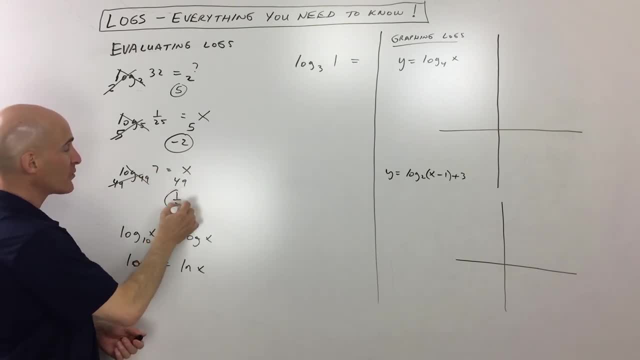 49 to what power is seven One half, because remember the one half power. that's like taking the square root. So the square root of 49 is seven. And then I just wanted to make a note here before I get to this. next one is that 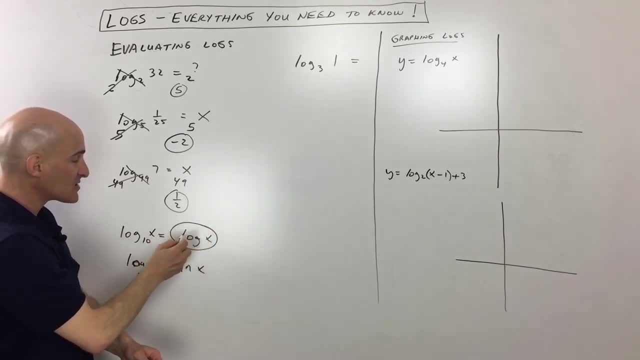 when you see log base 10 of x, a lot of times they're just gonna write it as log x. They won't even write a base here. It's called a common logarithm. It's kind of a lazy man's way of just writing log base 10 of x. 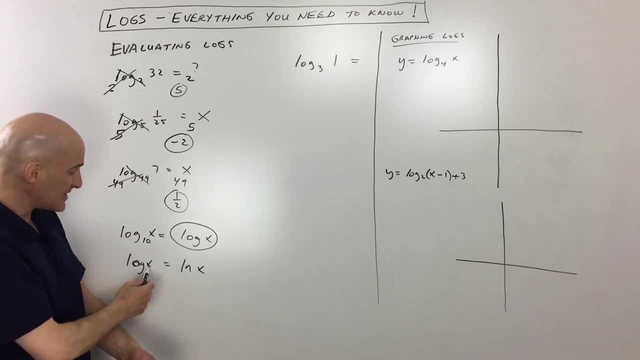 You'll see that on your calculator, log x, but that's base 10.. And then log base e of x. remember, e is the natural base e 2.71,. right, They'll write that as ln x or natural log of x. 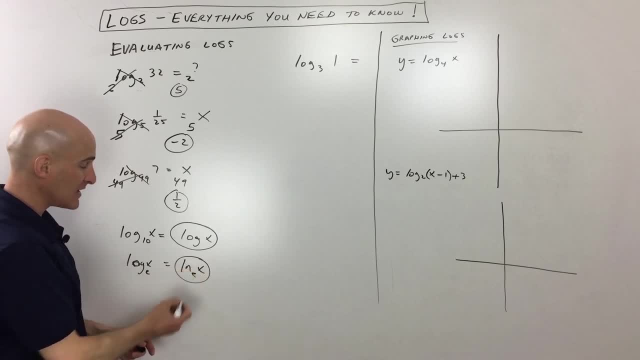 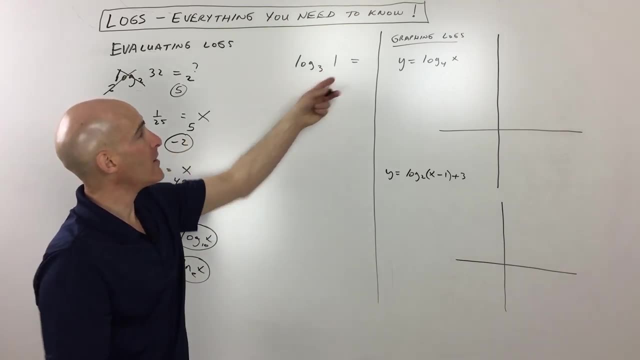 So these are like shorthand. So if you see that, if you want, you can put an e there to remind yourself, or a base 10 there again to remind yourself what base it is. So for this one log, base, three of one. 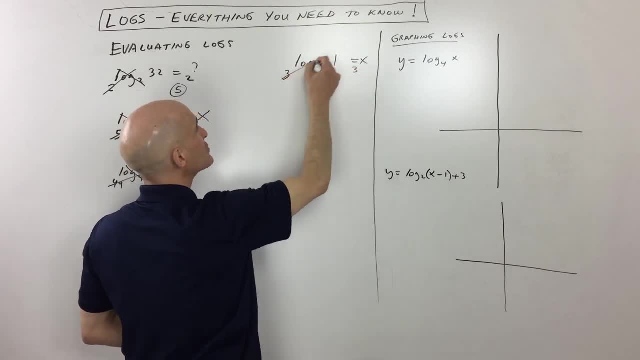 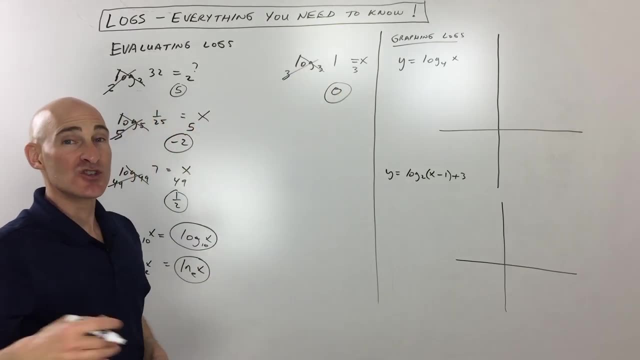 again, we're just gonna make it equal to x. So let's exponentiate both sides. These are inverses Three: to what power is one? Well, anything to the zero. power is one. so that's just gonna be zero. So now let's get into the graphing. 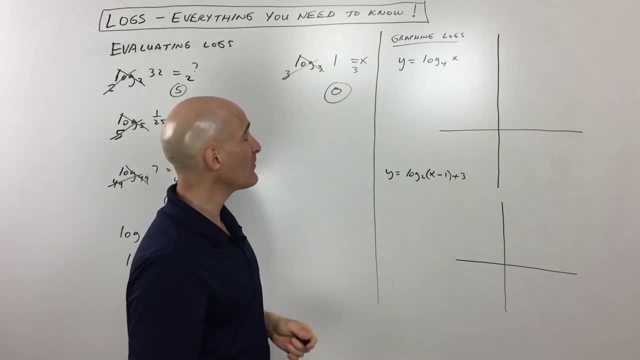 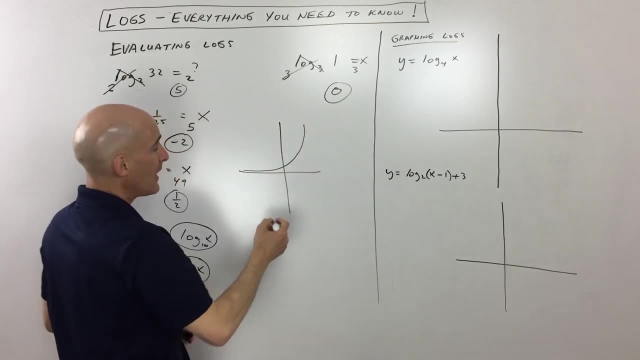 So how do you graph a log? okay? Well, here's the thing: We know that exponential functions which look like something like this- this is an exponential growth function and logarithmic functions are inverses. But when you wanna find the inverse of a graph, 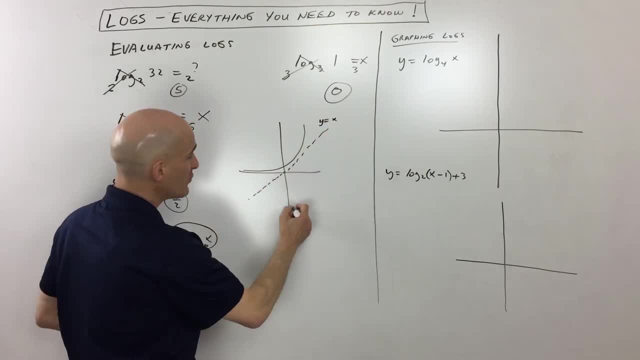 what you do is you reflect it over the line y equals x. So if we do that, the logarithmic graph should look something like this: right here Now the exponential graph: notice it's getting closer and closer to the x-axis, whereas the logarithmic graph is getting closer and closer. 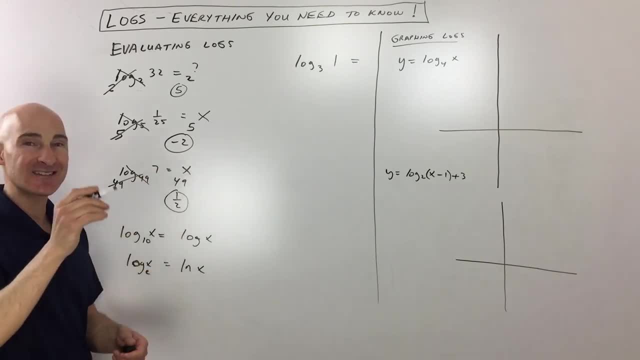 one half, because remember the one half power. that's like taking the square root, so the square root of 49 is 7. and then i just wanted to make a note here before i get to this. next one is that when you see log base 10 of x, a lot of times they're just going to write it as log x they. 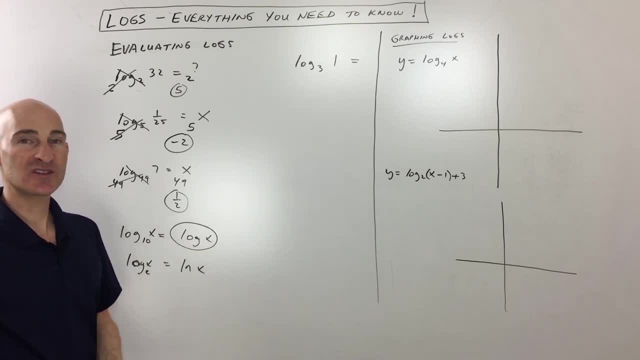 won't even write a base here. it's called a common logarithm. it's kind of a lazy man's way of just you know writing log base 10 of x. you'll see that on your calculator log x, but that's base 10. and then log base e of x. remember, e is the natural base, e 2.71. right, they'll write that as ln, x or. 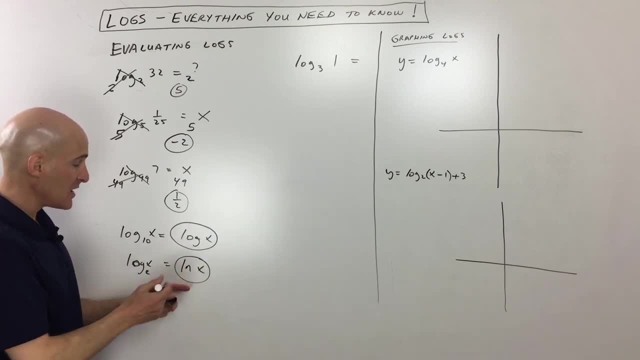 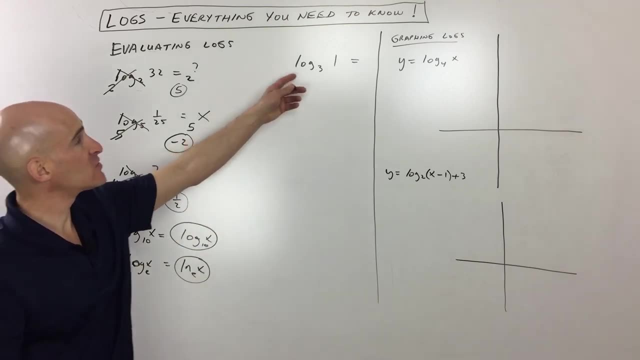 natural log of x. so these are like shorthands. so if you see that, if you want, you can put an e there to remind yourself, or a base 10 there again to remind yourself what base it is. so for this one log, base 3 of 1. 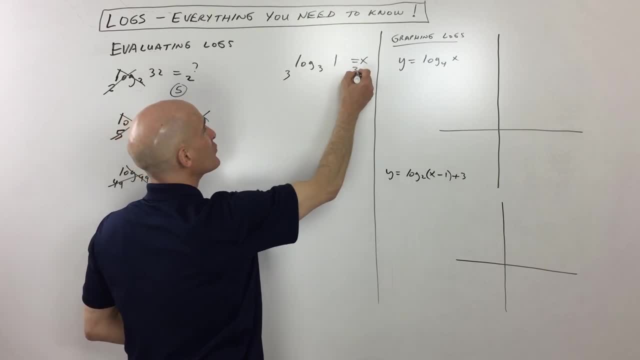 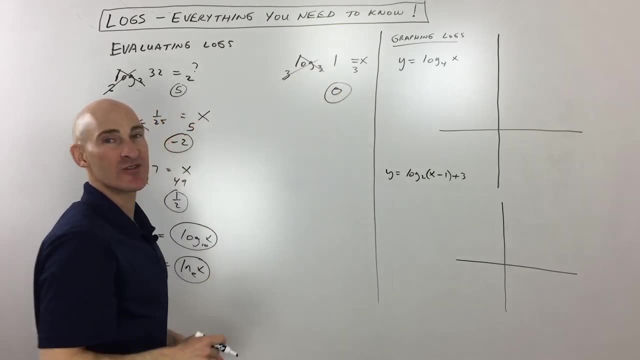 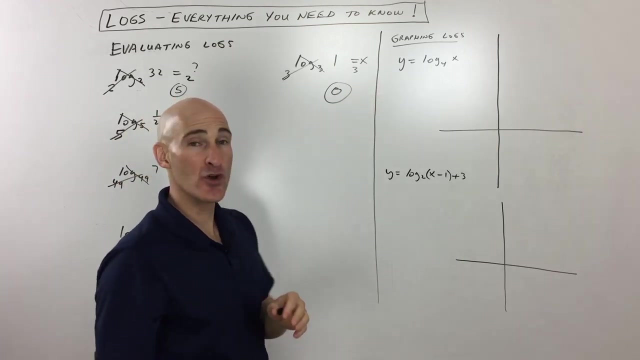 again, we're just going to make it equal to x. let's exponentiate both sides. these are inverses. 3 to what power is 1? well, anything to the 0 power is 1, so that's just going to be 0. so now let's get into the graphing. so how do you graph a log? okay, well, here's the thing. we know that. 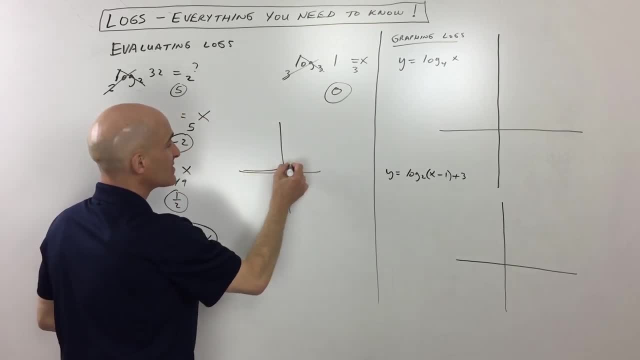 exponential functions which look like something like this: this is an exponential growth function and logarithmic functions are inverses. but when you want to find the inverse of a graph, what you do is you reflect it over the inverse of a graph and you're going to find the inverse of a graph. 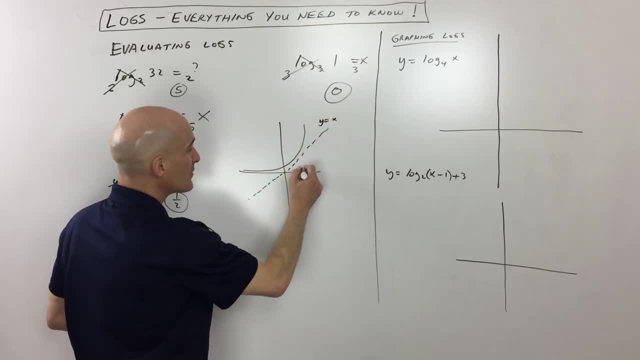 over the line y equals x. so if we do that, the logarithmic graph should look something like this right here now: the exponential graph- notice- is getting closer and closer to the x-axis, whereas the logarithmic graph is getting closer and closer to the y-axis. so this is going to be: 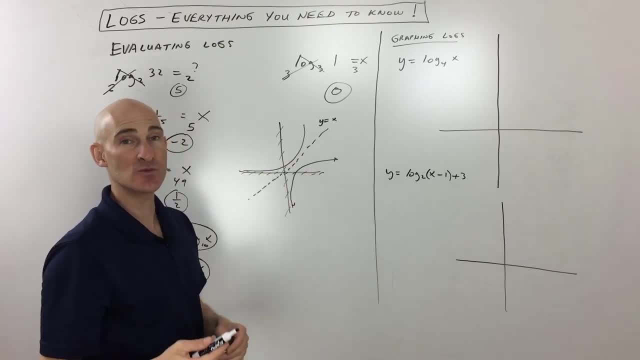 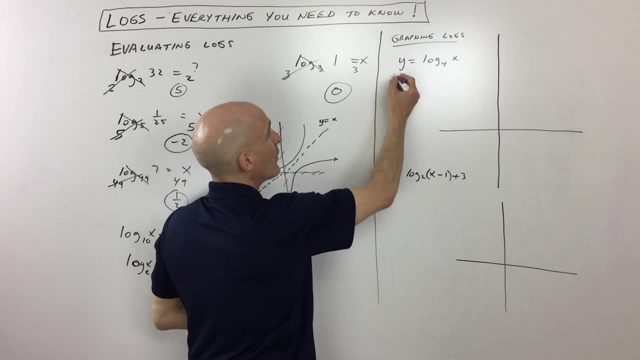 our vertical asymptote, as opposed to when we had the horizontal asymptote. let's go through some examples so you can see what i mean. so when you have y equals log base 4 of x, you want to graph that? what i would do, what i recommend, is just exponentiating both sides. okay, so i'm going to. 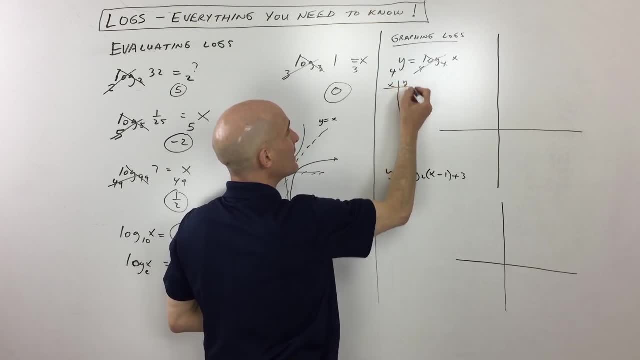 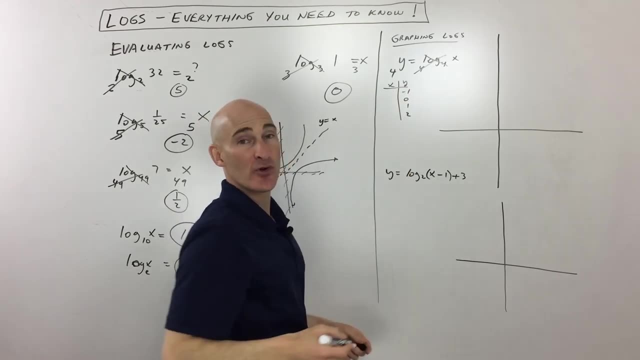 show you how to do that, okay. so now what we've done is we've rewritten it in exponential form. so we've got: x equals 4 to the y power. pick some values for y now, as opposed to x, because it's a little bit easier to take 4 to the negative 1, that's going to be 1. 4th 4 to the 0 is 1. 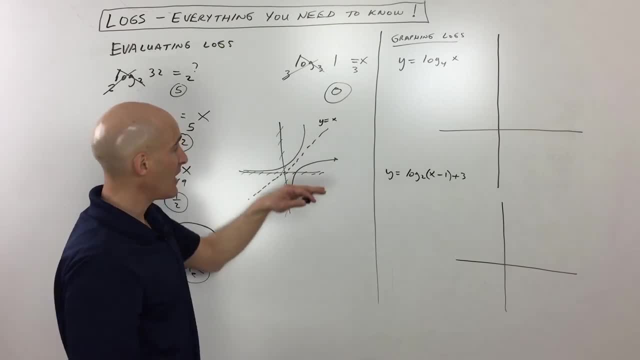 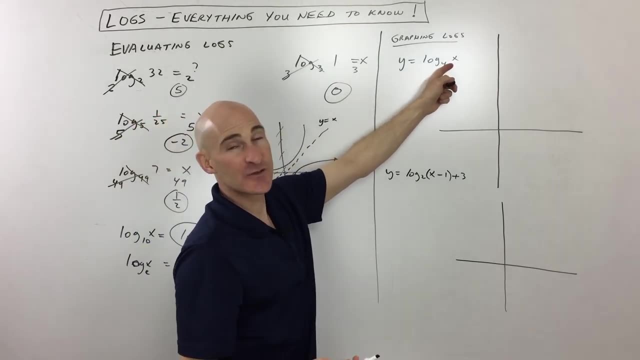 to the y-axis. so this is gonna be our vertical asymptote, as opposed to when we had the horizontal asymptote. Let's go through some examples so you can see what I mean. So when you have y equals log base four of x. 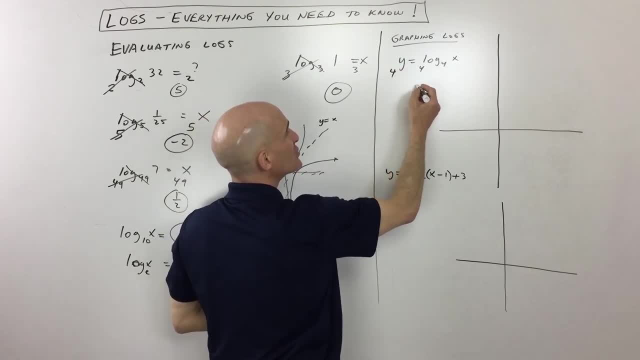 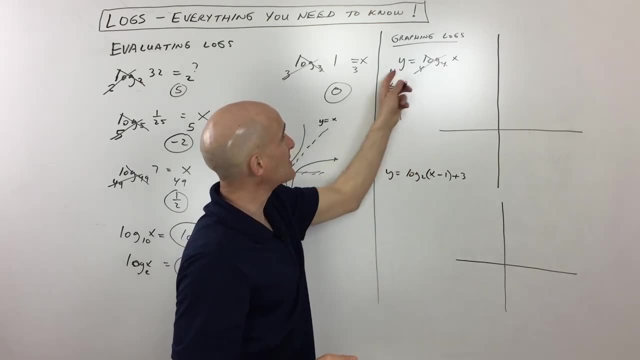 you wanna graph that? What I would do, what I recommend, is just exponentiating both sides. okay, So now what we've done is we've rewritten it in exponential form. So we've got x equals four to the y power. Pick some values for y now, as opposed to x. 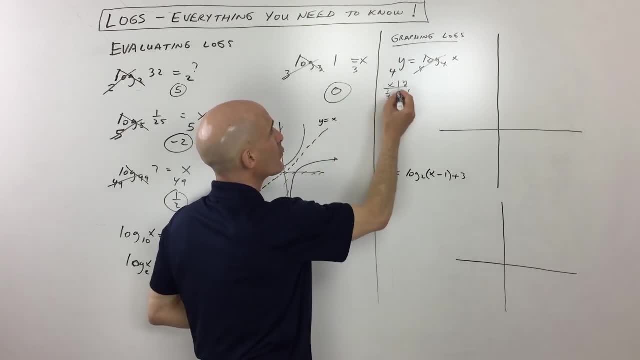 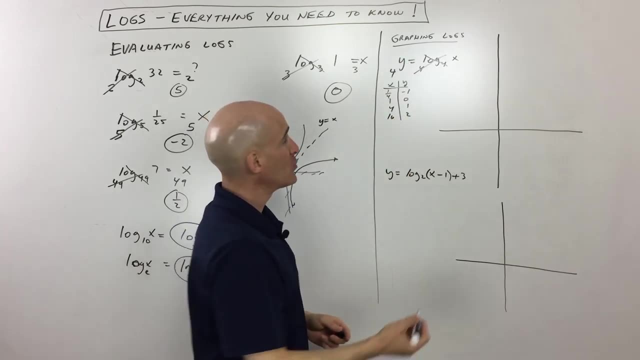 because it's a little bit easier to take four to the negative one. that's gonna be 1. 4th, four to the zero is one, four to the first is four and four to the second. power is 16.. Now what we can do is we can plot those points. 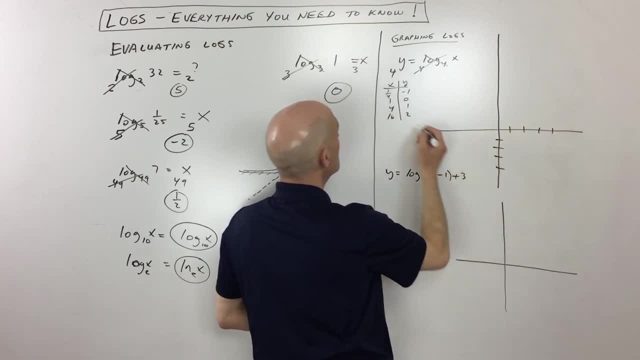 So we've got, let's see, when x is 1- 4th, we're going down one. when x is one, we're going right zero, and when we're going right four, we're going up one, and if we go way over here, 16,. 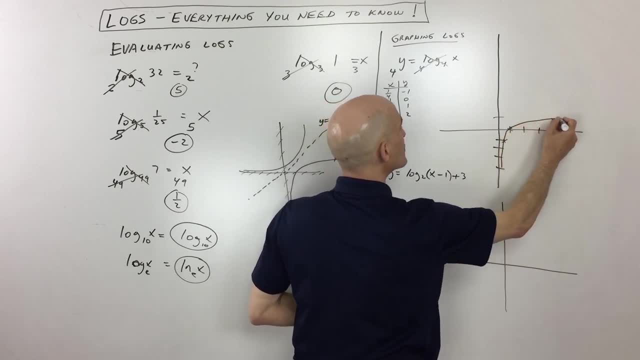 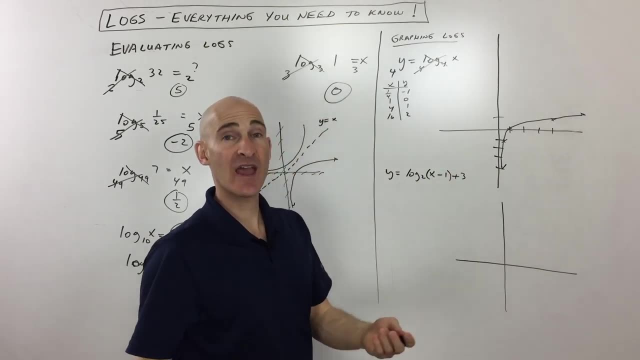 we're gonna be up at two, So I'm kind of going off the graph there, but our graph's gonna look something like that. Okay, so now the next thing your teacher might ask you is: you know what's the equation of the asymptote? 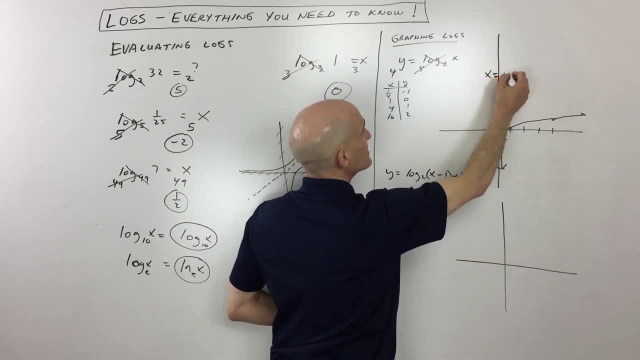 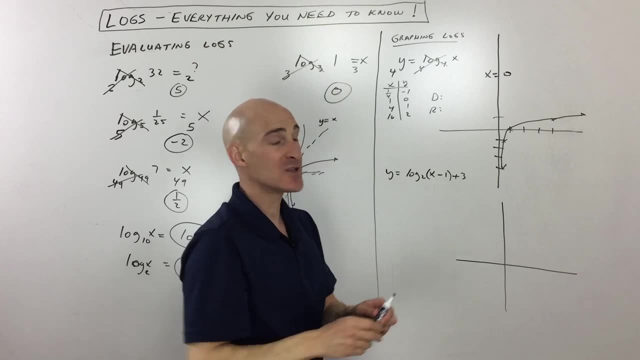 Well, because this is approaching the y-axis, that's actually the line. x equals zero, So that's your vertical asymptote. They might also ask you: what's the domain and the range? Well, remember, the domain is whatever the x value is. 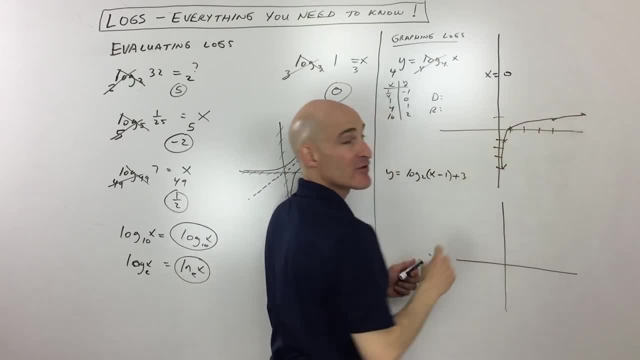 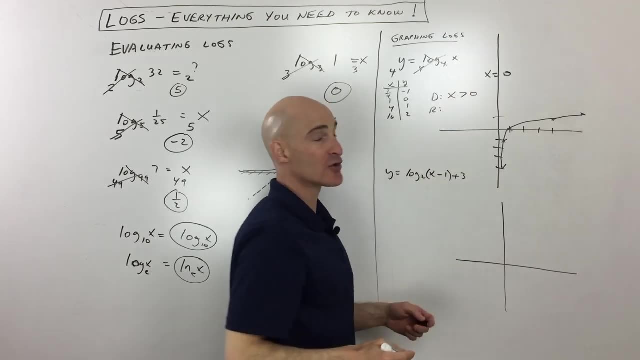 It can be, and in this case x is greater than zero. You don't see the graph over here in the negative range. It's not touching the y-axis, so x can't be zero. So the domain is x is greater than zero. 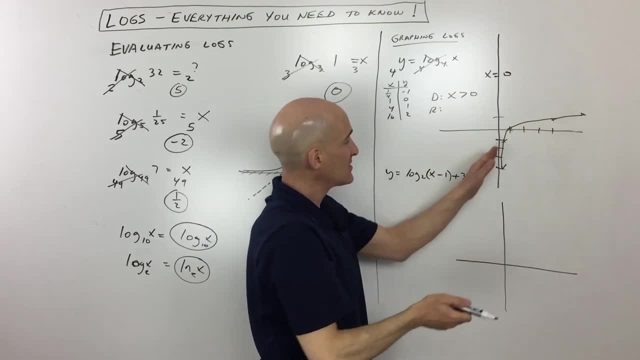 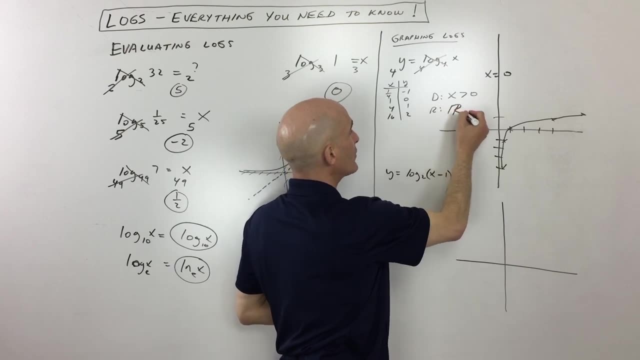 and then for the range, we think about what the y values are and you can see this is going down towards negative infinity, gradually making its way up towards positive infinity. so the range is gonna be all real numbers. okay, Let's do a little bit more complicated example. 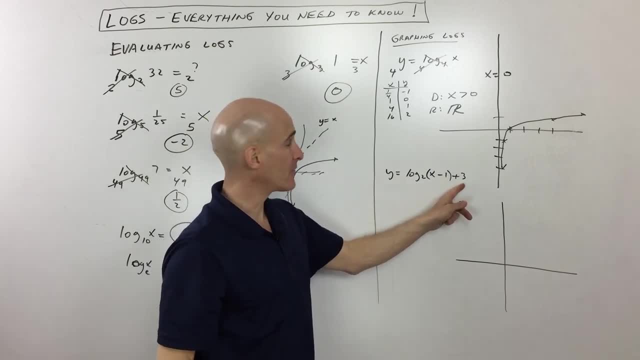 So this one here. what do you think the one and the three do to the graph? Well, the number that's grouped with the x, it shifts the graph in the x direction, the horizontal direction. but this minus one has the opposite effect. 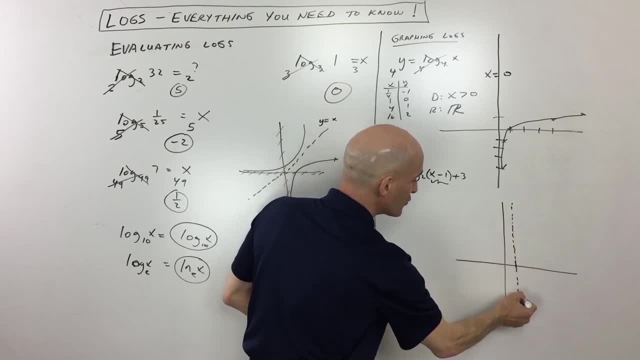 It's actually gonna shift it right one, so we actually have a vertical asymptote here at x equals one. okay, and then what do you think the positive three does? Well, it shifts it up three, so we can think of this point. 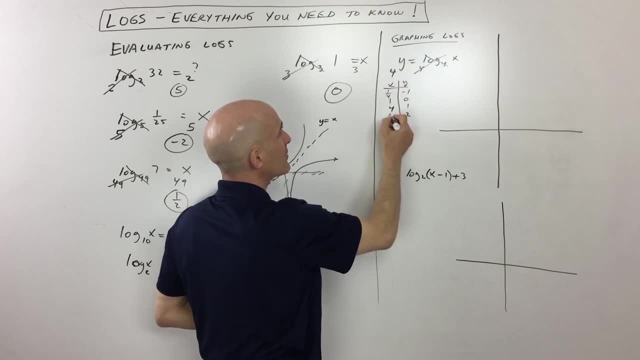 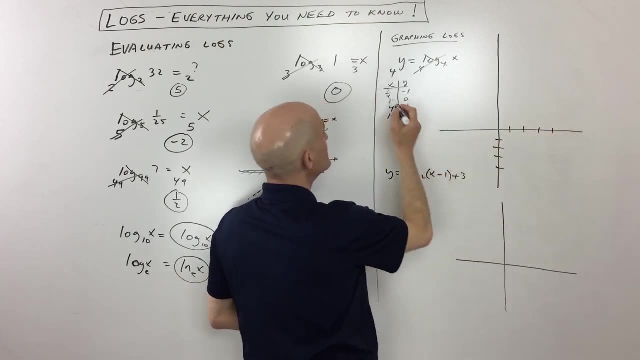 4 to the first is 4 and 4 to the second, power is 16. now what we can do is we can plot those points. so we've got, let's see, when x is 1, 4th, we're going down 1, and x is 1, we're going right 0, and when we're going right 4, we're going up 1, and if we go way, 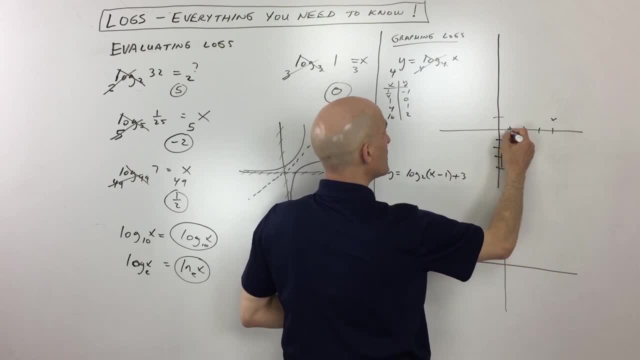 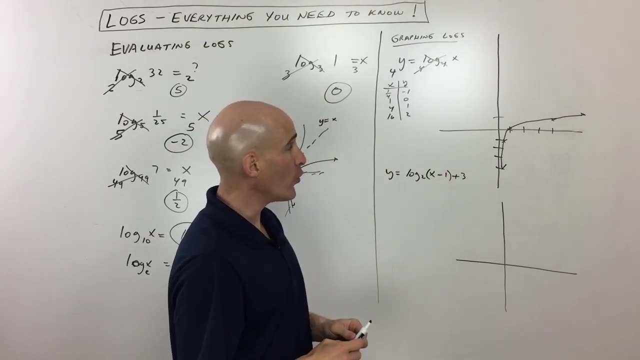 over here 16. we're going to be up at 2, so i'm kind of going off the graph there, but our graph's going to look something like that. okay, so now the next thing your teacher might ask you is: you know what's the equation of the asymptote? well, because this is approaching the y-axis. that's actually the line. 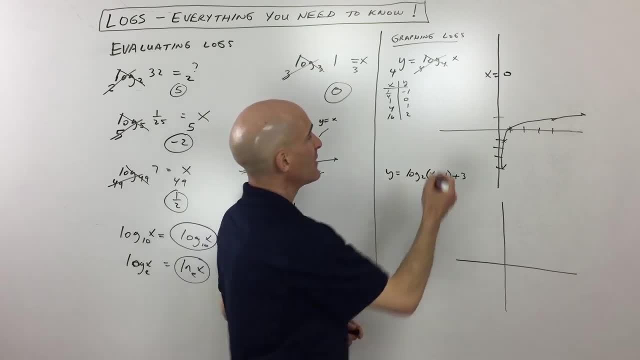 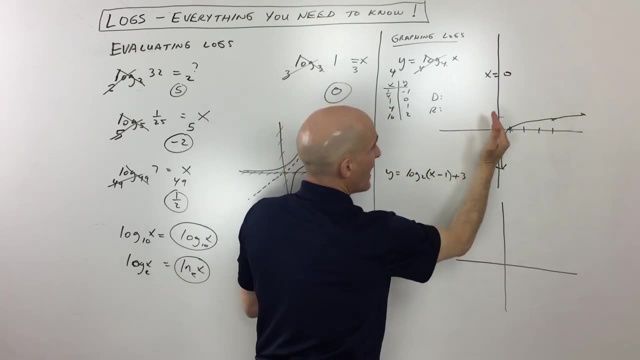 x equals 0. so that's your vertical asymptote. they might also ask you: what's the domain? in the range, the domain is whatever the x values can be, and in this case x is greater than 0. you don't see the graph over here. in the negative range it's not touching the y-axis, so x can't be 0. so the domain: 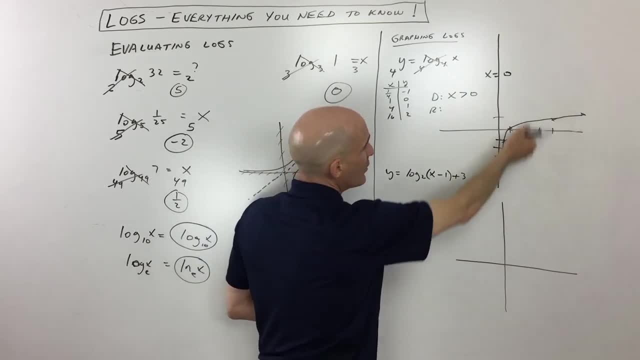 is x is greater than 0, and then for the range, we think about what the y values are and you can see this is going down towards negative infinity, gradually making its way up towards positive infinity. so the range is going to be all real numbers. okay, let's do a little bit more complicated. 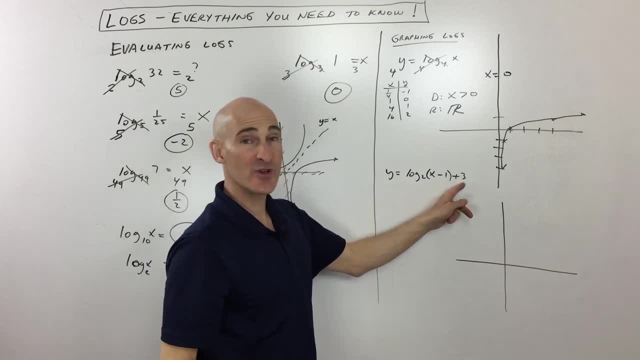 example. so this one here. what do you think the 1 and the 3 do to the graph? well, the number that's grouped with the x, it shifts the graph in the x direction, the horizontal direction. but this minus 1 has the opposite effect. it's actually going to shift it right. 1, so we 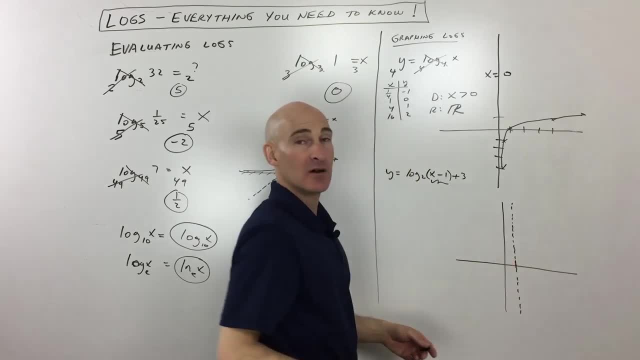 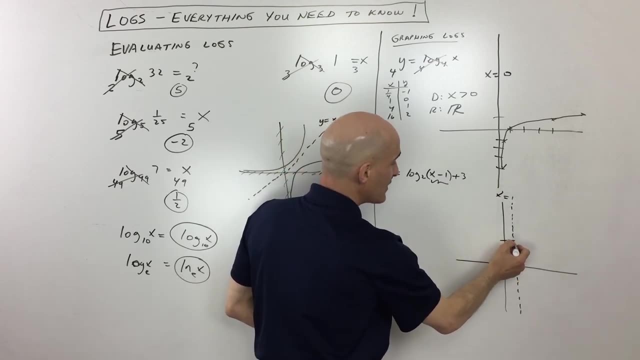 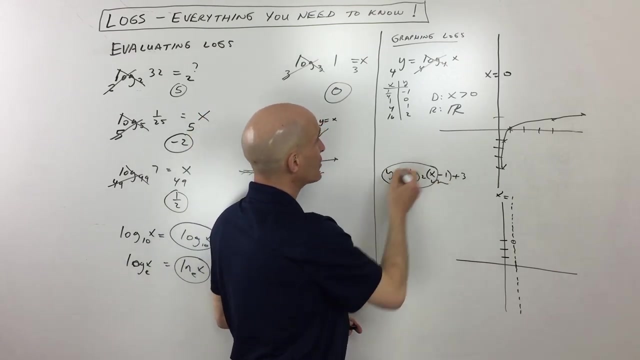 actually have a vertical asymptote here: at x equals 1. okay, and then what do you think the positive 3 does? well, it shifts it up 3, so we can think of this point right here, that circle that I drew as our origin, as our starting point. now we're just going to focus on the parent function. okay, y. 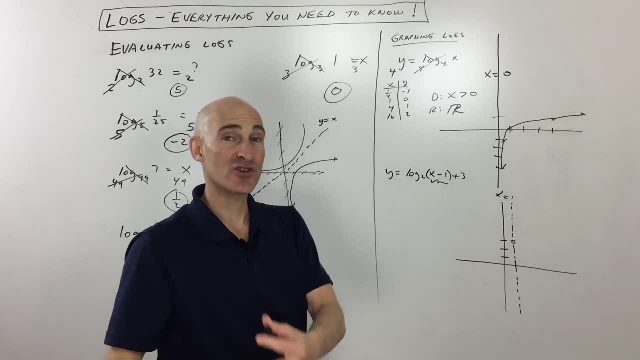 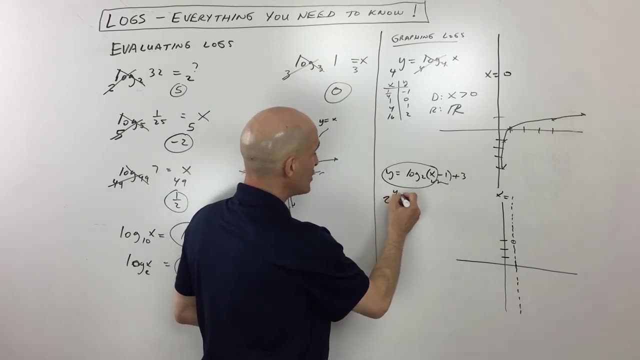 right here that circle that I drew as our origin, as our starting point. Now we're just gonna focus on the parent function. okay, y equals log base two of x. We're gonna exponentiate both sides. okay, These are inverses, so we get two to the y equals x. 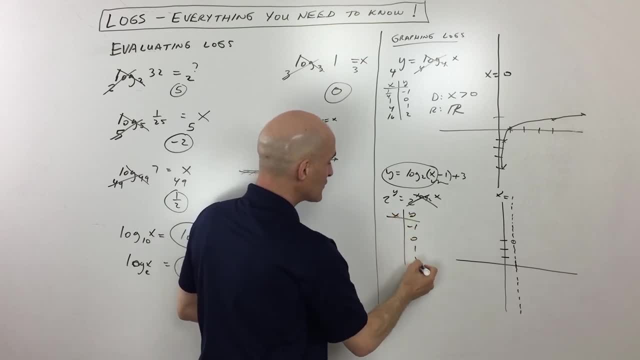 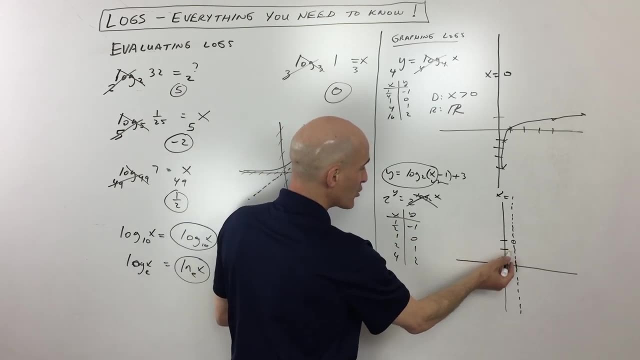 So I'm gonna make a table again, I'm gonna plug in some easy values for y. so this is gonna give us one, half, one, two and four, and then what I'm gonna do is I'm gonna plot the points from here, not the origin, because everything's shifting. 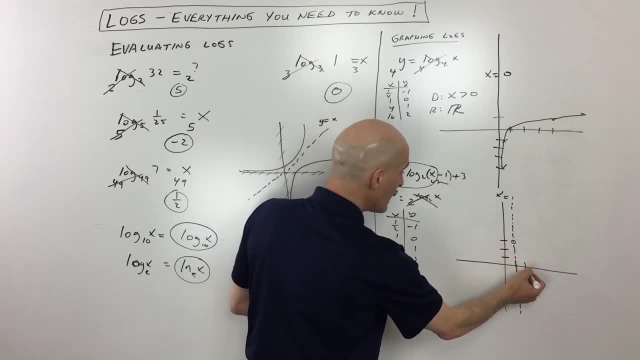 right one up three anyways. so let's just start from here And let's see. so if we go right a half down one, that'd be right there. Right one: Okay, up zero. and then right two, Okay, let's see: right two up one, like that. 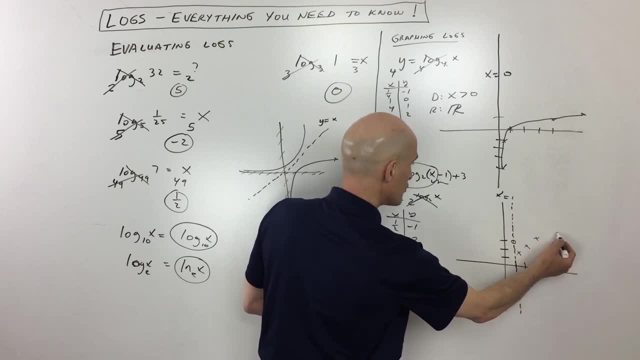 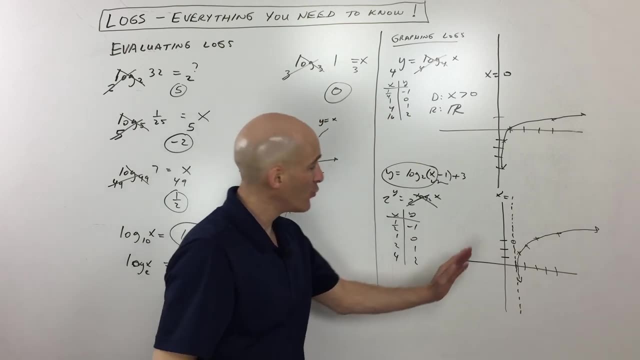 and then right four, one, two, three, four up two, so something like that. So basically, this graph looks something like that: all right, and you can see the domain is gonna be, x is greater than one and the range is gonna be. 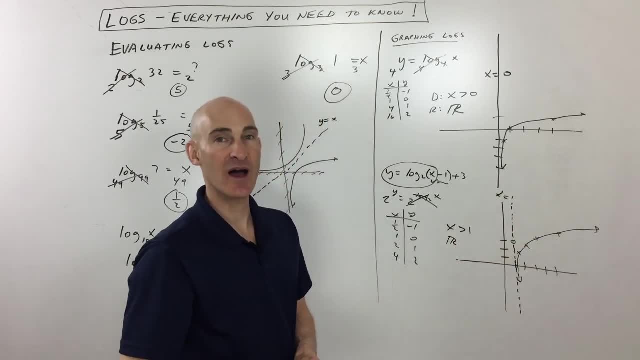 all real numbers, so it's going up and down from negative infinity to positive infinity. Okay, so that's talking about the graphing. The next thing we're gonna talk about is expanding and condensing logs. so let me erase this board and we'll do that next. 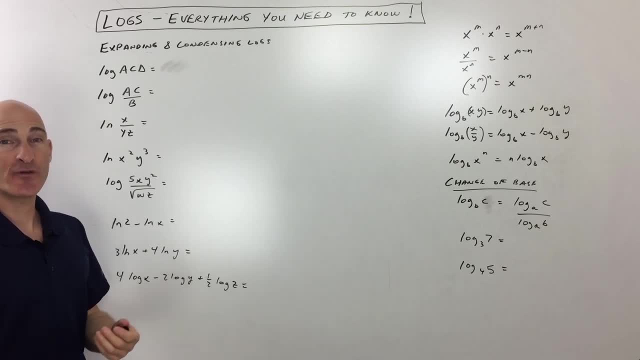 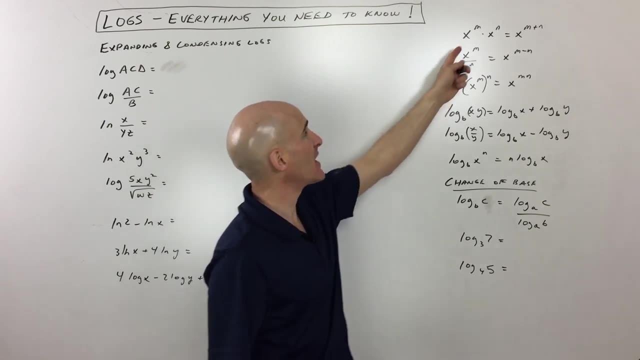 Okay, now we're gonna talk about expanding and condensing logs, but first we wanna talk about the properties of logs. okay, Just like there's properties of exponents, rules of exponents. for example, when you multiply and you have the same base, what do you do to the exponents? 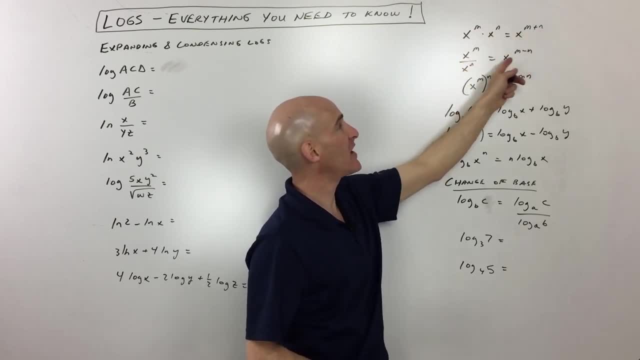 You add them right. When you divide and you have the same base, what do you do to the exponents? You subtract them. What do you do when you have a power to power? You multiply. so those are the rules of exponents. 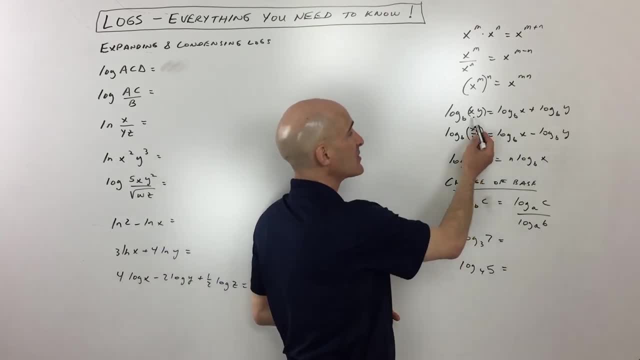 you learned before The rules of logs. it's very similar. When you have these two arguments multiplied together, you can write it as a sum of two logs. The main thing is you wanna make sure that you keep the base the same, whatever that base is. 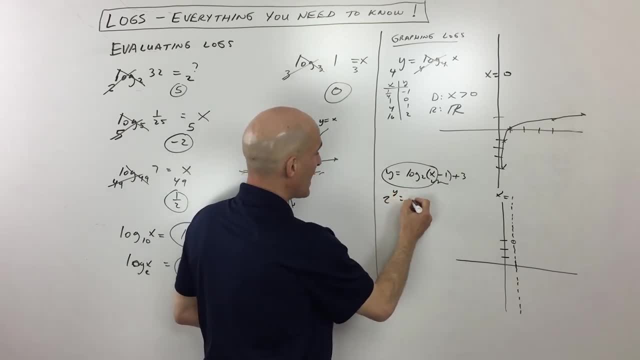 2 of x. we're going to exponentiate both sides. okay, these are inverses. so we get 2 to the y equals x. so I'm going to make a table again. I'm going to plug in some easy values for y. so this is going. 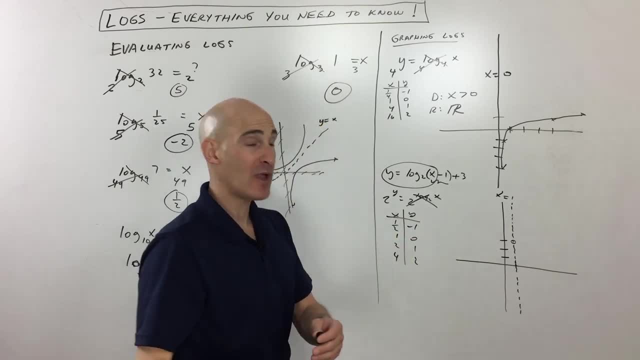 to give us one half, 1, 2 and 4, and then what I'm going to do is I'm going to plot the points from here, not the origin, because everything's shifting right. 1 and up, 3 anyways. so let's just start from. 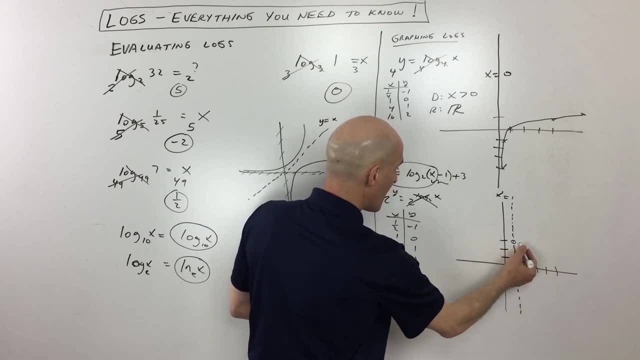 here and let's see. so if we go right a half down 1, that'd be right there. right 1: okay, up 0, and then right 2. okay, let's see right 2, up 1, like that, and then right 4: 1, 2, 3, 4. 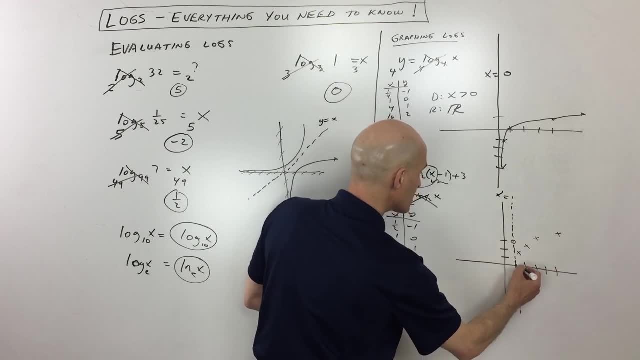 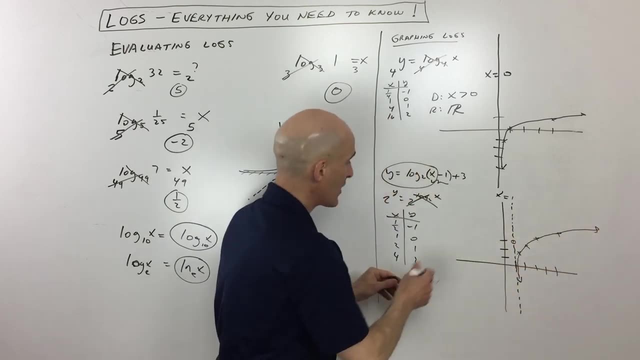 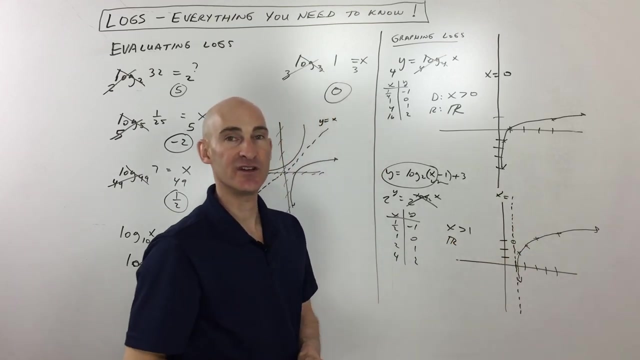 up 2, so like something like that. so basically this graph looks something like that, all right, and you can see the domain is going to be x is greater than 1 and the range is going to be all real numbers. so it's going up and down from negative infinity to positive infinity, okay, so. 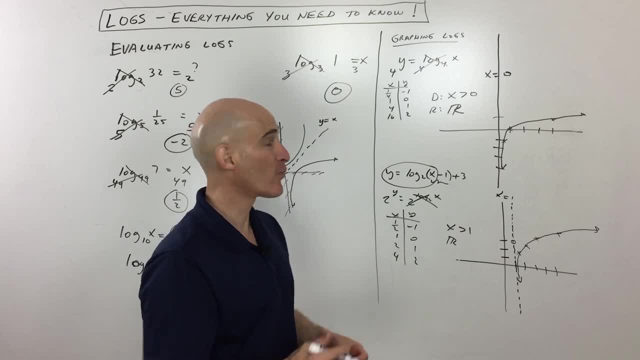 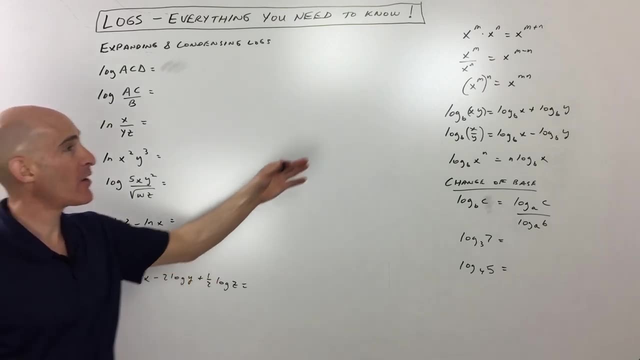 the next thing we're going to talk about is expanding and condensing logs, so let me erase this board and we'll do that next. okay, now we're going to talk about expanding and condensing logs, but first we want to talk about the properties of logs. okay, just like those properties of exponents. 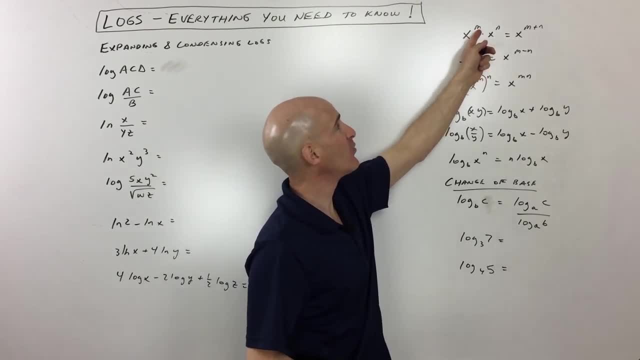 rules of exponents. for example, when you multiply and you have the same base, what do you do to the exponents? you add them right. when you divide and you have the same base, what do you do to the exponents? you subtract them. what do you do when you have a power to power? you multiply, so those 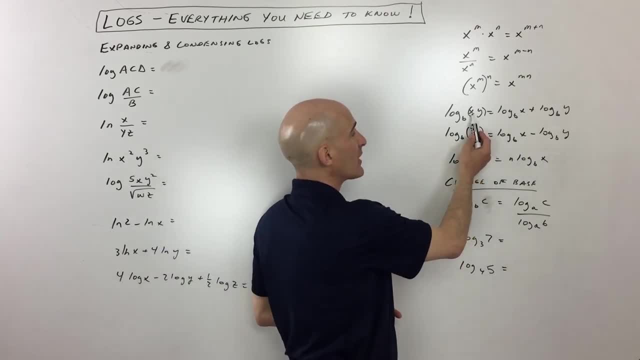 four. but now the rules of logs. it's very similar, like when you have these two arguments multiply together, you can write it as a sum of two logs. the main thing is you want to make sure that you keep the base the same. whatever that base is, same thing over here. if you're dividing these, 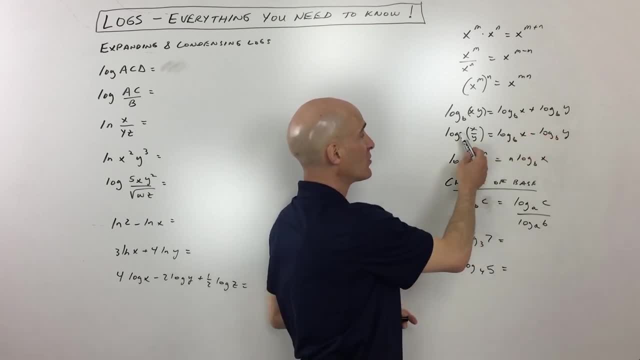 two arguments. you can write it as a difference of two logs. just take the log of the numerator minus the log of the denominator, and then this one's called the power property. you can take this exponent here and you can bring it down in front and write it as a coefficient. 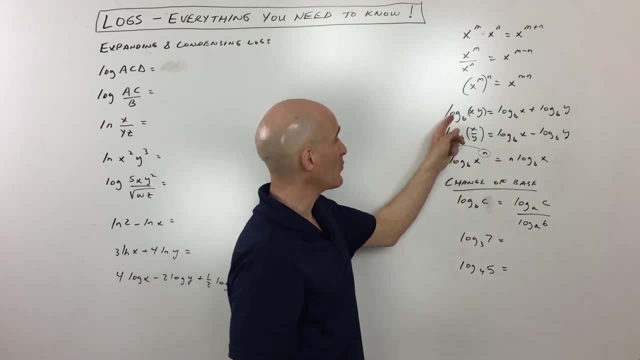 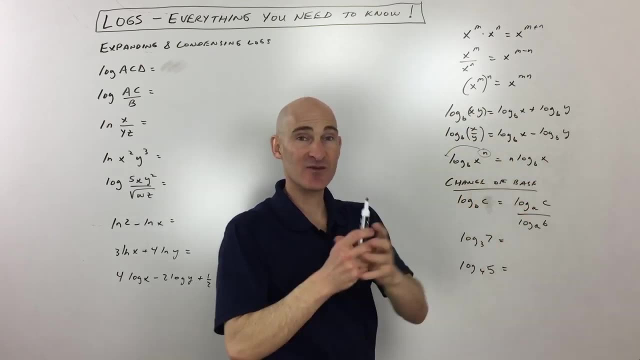 now all these properties. they're reversible. so when you're going from the left to the right, that's called expanding- it's getting larger. but if you go from the right to the left, that's called condensing- it's getting feel more condensed right. so if you see the sum of two logs, you can write it. 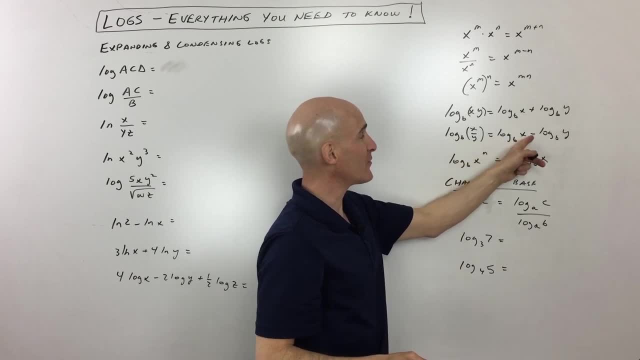 Same thing over here. If you're dividing these two arguments, you can write it as a difference of two logs. Just take the log of the numerator minus the log of the denominator, and then this one's called the power property. You can take this exponent here. 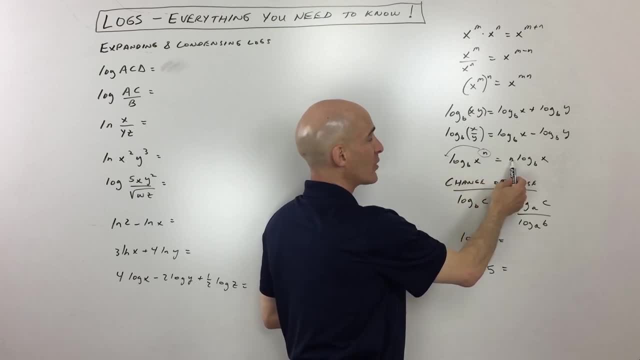 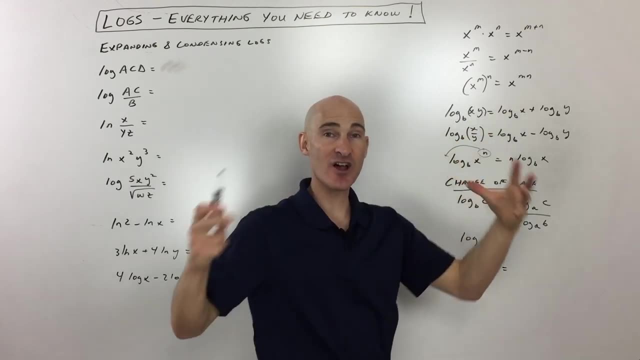 and you can bring it down in front and write it as a coefficient. Now, all these properties, they're reversible. so when you're going from the left to the right, that's called expanding. It's getting larger. but if you go from the right to the left, 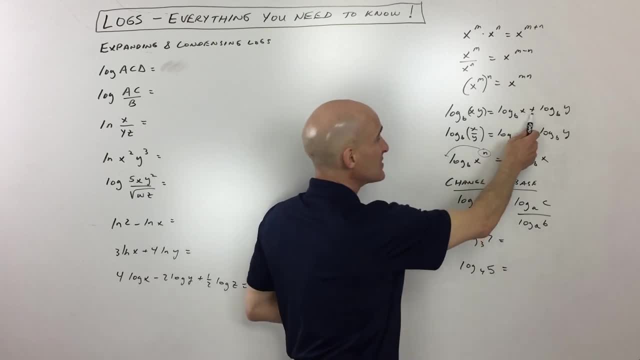 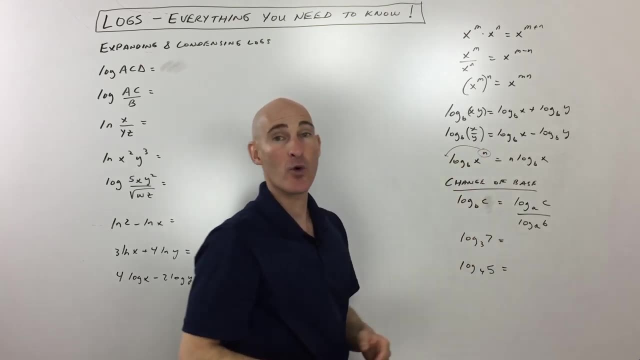 that's called condensing. It's getting more condensed, right? So if you see the sum of two logs, you can write it as log of a product. or if you see the difference of two logs and they have the same base, you can write it as the log of a quotient. okay. 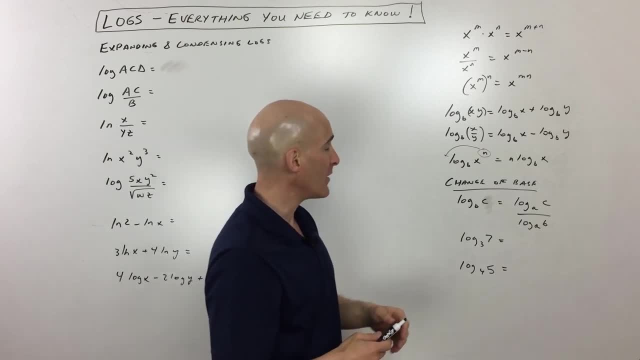 And then there's another formula called the change of base formula, and this really comes in handy when some calculators they don't have the ability to change the base. They only have log base 10, log which is log base E. So what you can do here is if you have log base B of C, 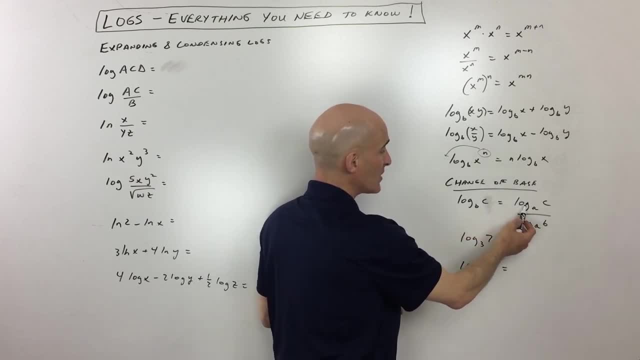 equals log. you pick a new base, let's say base A. you take log base A of C divided by log base A of B. So, for example, if you had log base three of seven, you could really write this as a common log. 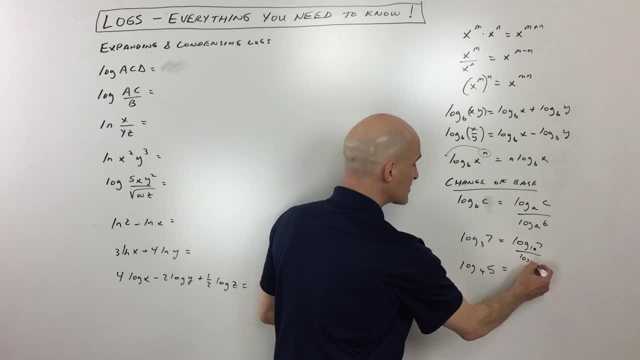 like log base 10 of seven divided by log base 10 of three. Now it's easy to remember because the seven's a little bit higher, that goes in the numerator, The three's a little bit lower, that goes in the denominator. 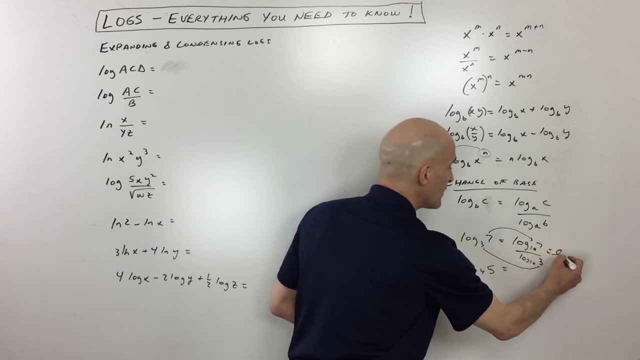 You just pick a new base and that's it. You can also write this as natural log of seven over natural log of three. Same thing with this one log base, four of five. I would just say natural log of five over natural log of four. 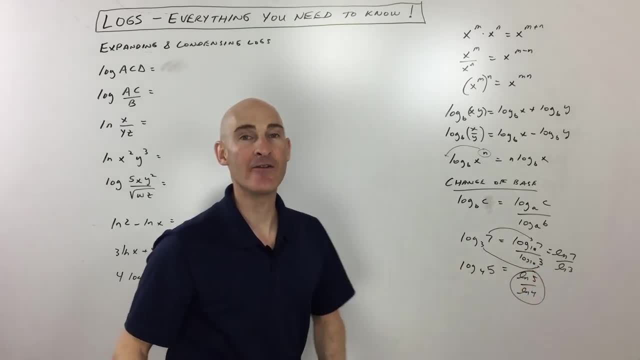 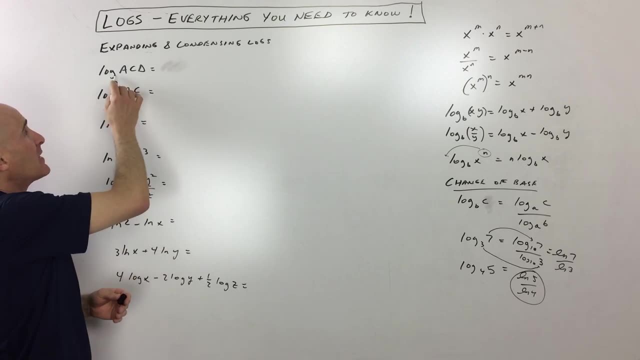 Put that in your calculator and you got the same thing as log base four of five. But let's get into the expanding and condensing now. So say you wanna expand log of A times C, times D. I didn't write the base there. 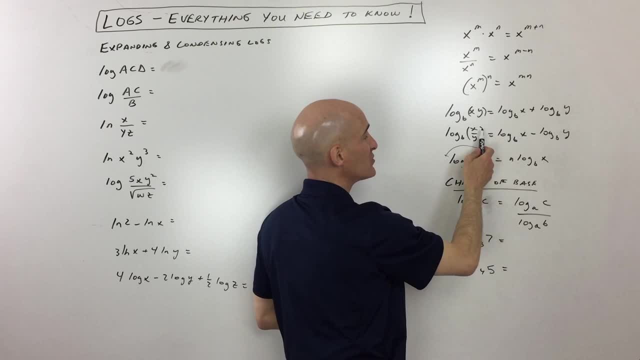 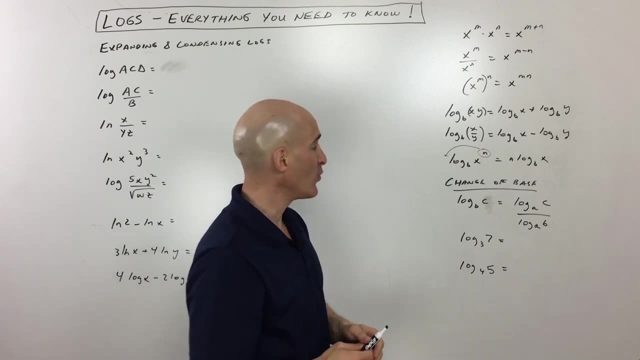 as log of a product, or if you see the difference of two logs and they have the same base, you can write it as the log of a quotient. okay, and then there's another formula called the change of base formula, and this really comes in handy when some calculators they don't have the ability to change. 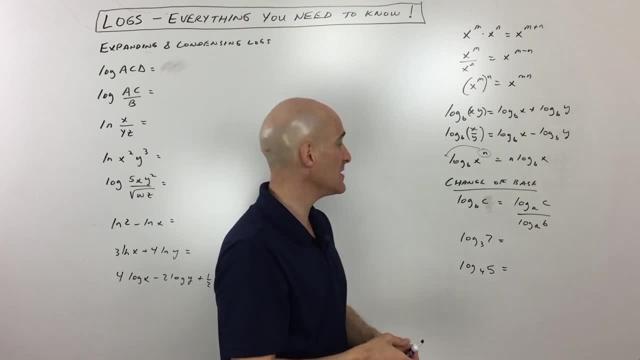 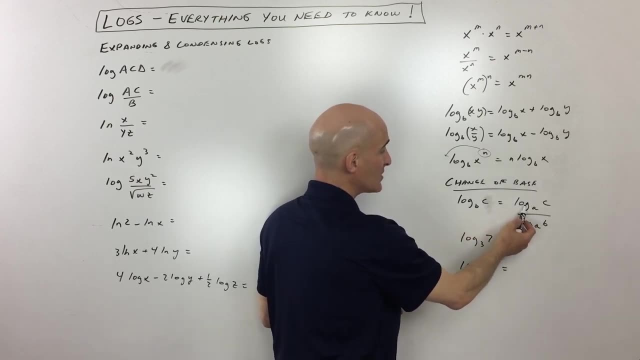 the base. they only have log base 10 or an astral log, which is log base e. so what you can do here is, if you have log base b of c equals log, you pick a new base, let's say base a. you take log base a of c divided by log base a of b. so 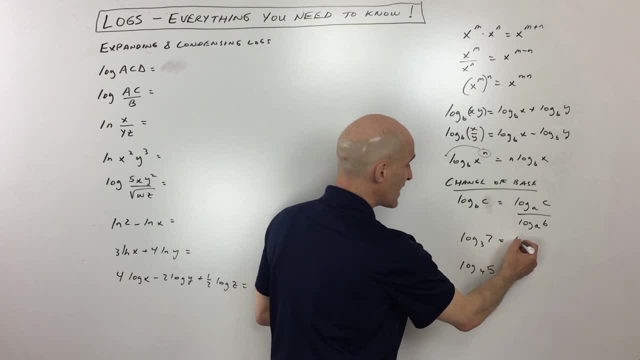 for example, if you had log base 3 of 7, you could really write this as a common log, like log base 10 of 7 divided by log base 10 of 3.. now it's easy to remember because the 7 is a little bit higher. 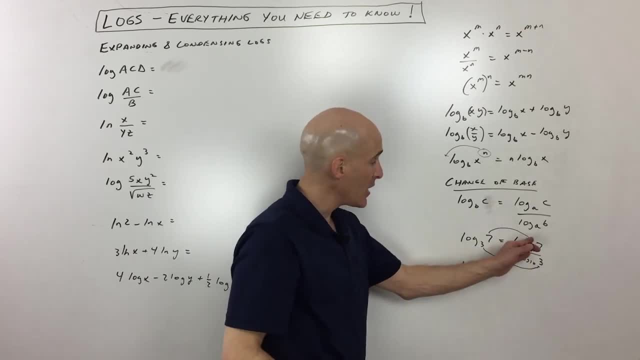 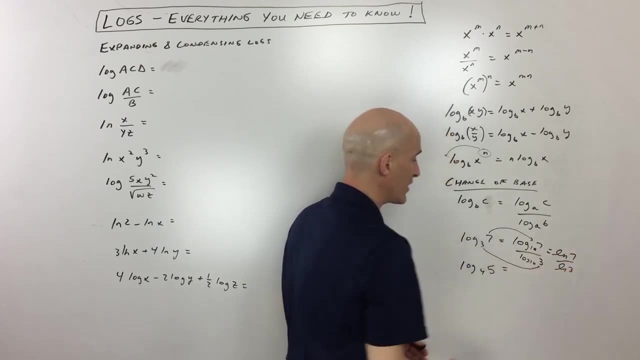 that goes in the numerator. the 3 is a little bit lower. that goes in the denominator. you just pick that is and that's it. you can also write this as natural log of 7 over natural log of 3.. same thing with this one log base, four or five. I would just say natural log a 5 over natural log of 4 put. 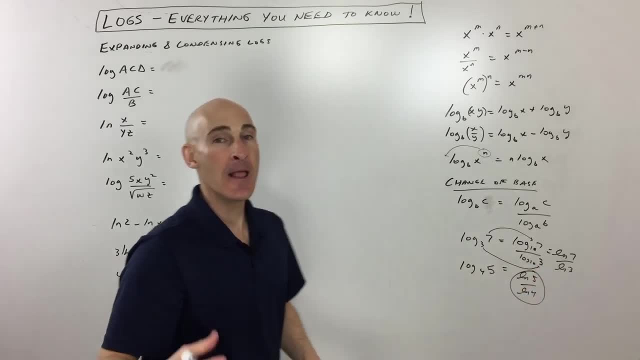 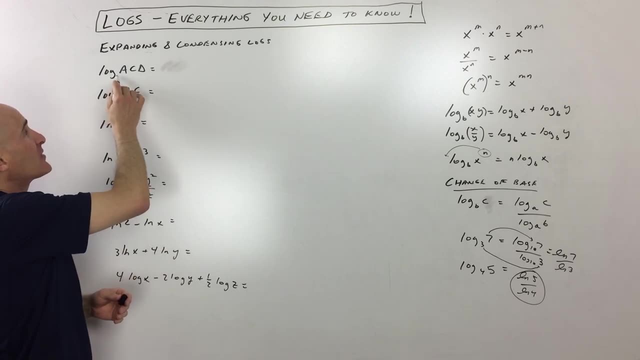 that in your calculator and you got the same thing as log base four or five. but let's get into the expanding and condensing now. so say you want to expand log of A times c, times D. I didn't write the base there, so that's considered a common log or log base 10. but because these are all multiplied, 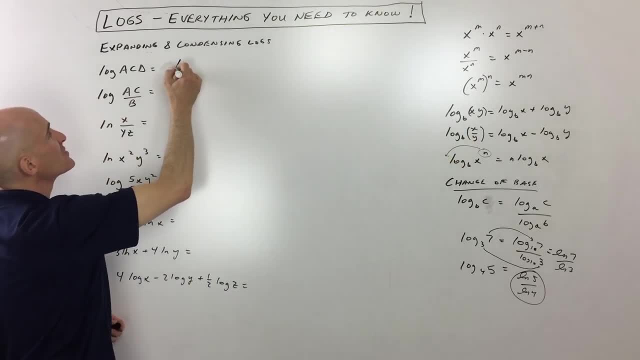 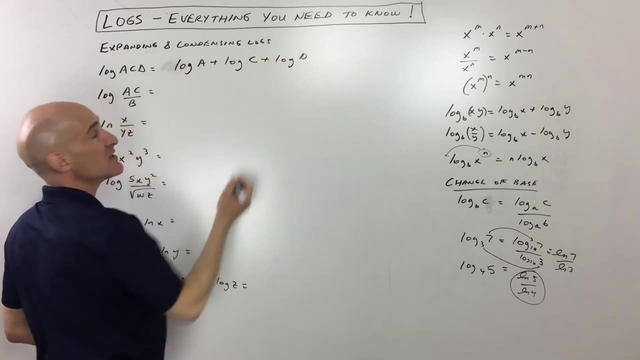 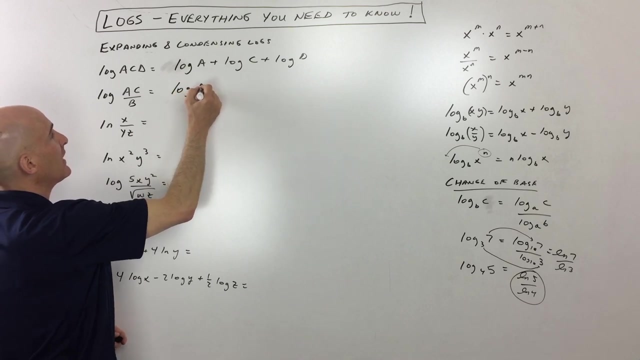 we're going to use the product okay rule. so this is going to be log of a plus log of C plus log of D. pretty easy, right here we've got a combination of multiplying and dividing. so what I'm going to do is I'm going to do log of a plus log of C minus log of B, so the one that I'm dividing by we're. 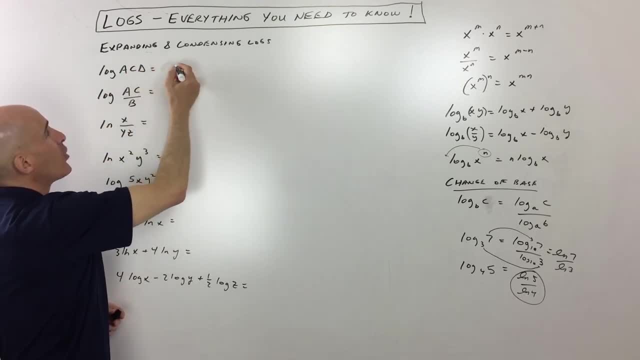 so that's considered a common log or log base 10.. But because these are all multiplied together, we're gonna use the product okay rule. So this is gonna be log of A plus log of C plus log of D. Pretty easy, right. 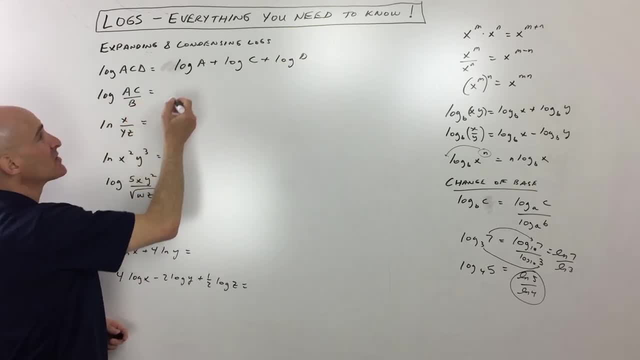 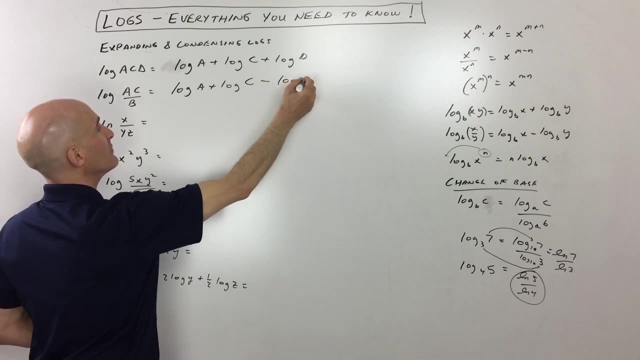 Here we've got a combination of multiplying and dividing. So what I'm gonna do is I'm gonna do log of A plus log of C minus log of B, So the one that I'm dividing by we're subtracting, The ones that are multiplied together we're adding. 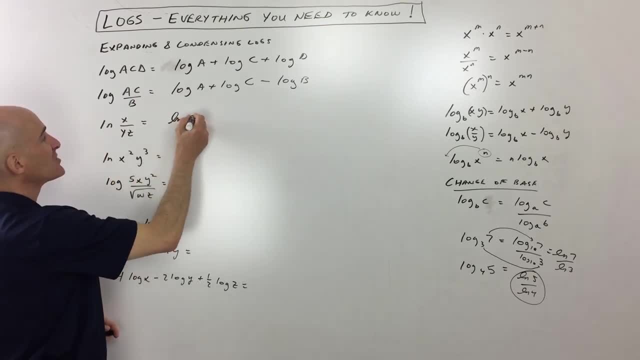 This one here natural log. this one's gonna be. I'm gonna do it in two steps. I'm gonna do natural log of A, natural log of B, natural log of D, Natural log of X minus- see, because we're dividing- natural log of Y times Z. 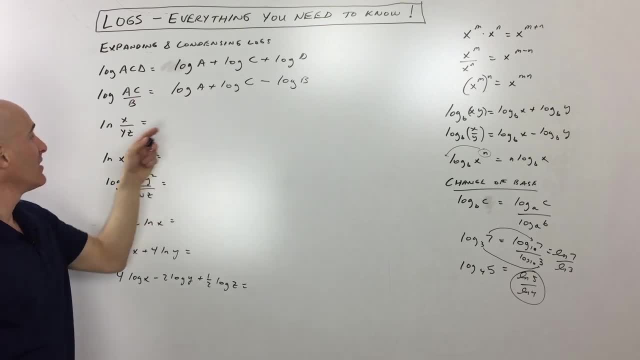 subtracting the ones that are multiplied together. we're adding this one here, natural log. this one's going to be. I'm going to do it in two steps. I'm going to do natural log of X minus C, because we're dividing natural log of Y times Z, but you can see these are multiplied together, which we can write. 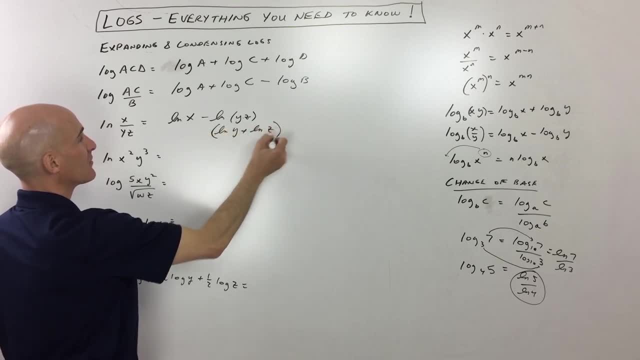 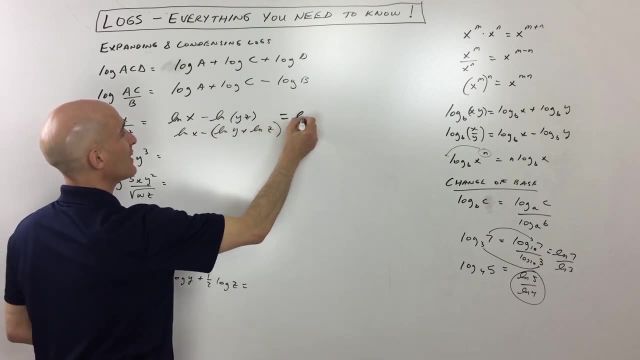 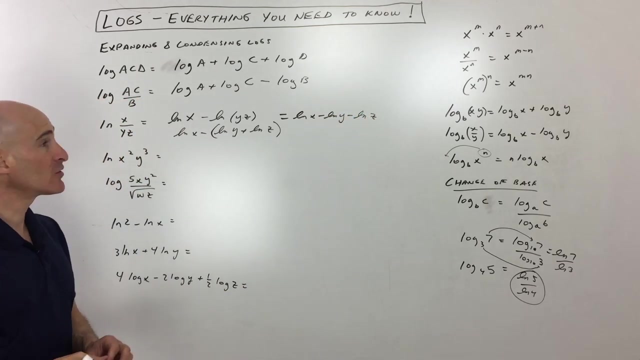 this as natural log of Y plus natural log of Z. right, but you see this whole thing is being subtracted so we have to distribute that negative. so this whole thing comes out to natural log of X minus natural log of Y minus natural log of Z. the thing to take away from this particular example is: whatever's in the 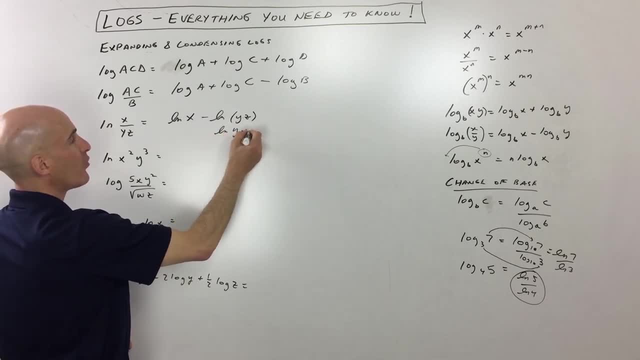 But you can see these are multiplied together, which we can write this as natural log of Y plus natural log of Z, right? But you see this whole thing is being subtracted so we have to distribute that negative. So this whole thing comes out to natural log of X. 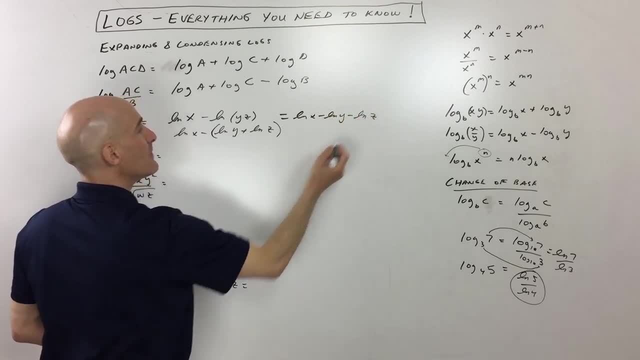 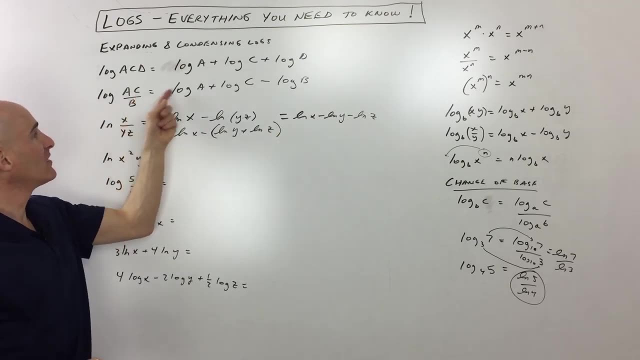 minus natural log of Y, minus natural log of Z. The thing to take away from this particular example is: whatever's in the denominator you're gonna be subtracting, Whatever's in the numerator is gonna be positive or you're gonna be adding: okay. 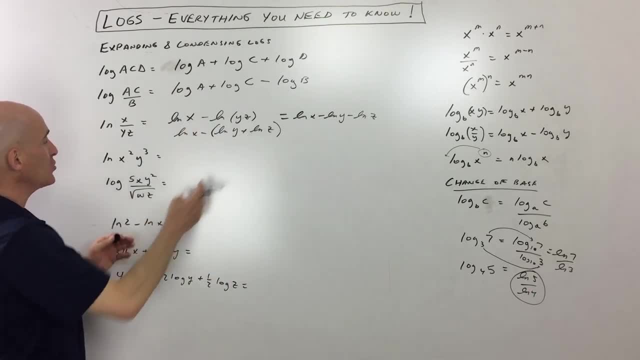 So that's just a quick way to figure these ones out, But you can do it in steps like this too. This one: we've got some exponents here, So this is actually gonna be natural log of X squared plus natural log of Y cubed. 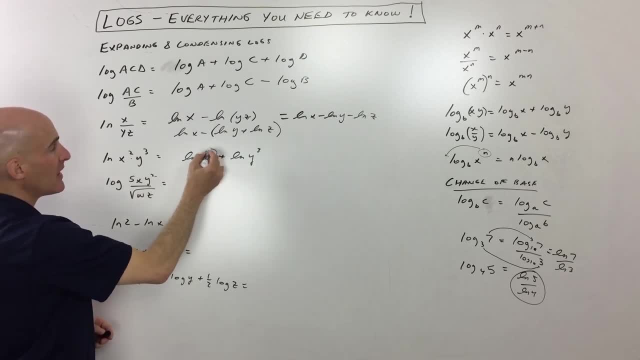 because you can see these are multiplied. so I wrote it as a sum of two logs. Then what I'm gonna do is I'm gonna bring those powers down in front as coefficients. That's the power property. okay for log. So this is gonna be two natural log of X. 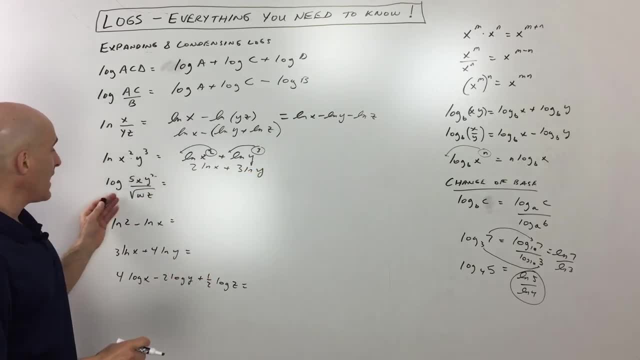 plus three natural log of Y. That's fully expanded. And then one here. this is a pretty more challenging one. Let's see it's log of. let's see log of five plus log of X plus two log of Y. 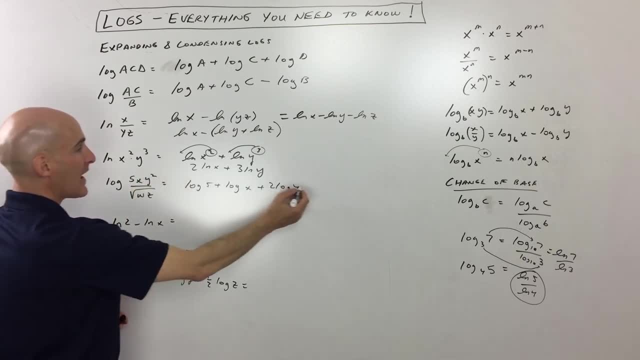 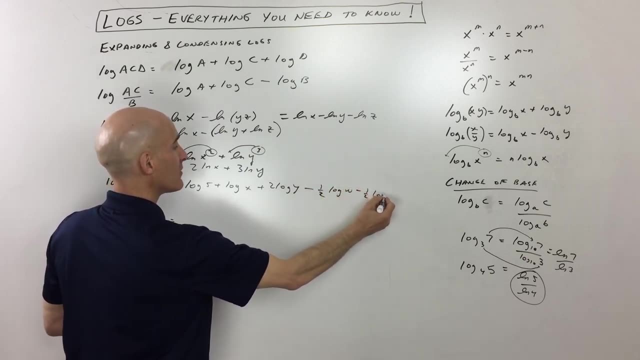 See, I brought down that two in front, okay, And then minus, because we're dividing one half log of W minus one half log of Z. So I did all that and then I did one step. Now you don't have to do it in one step like I did. 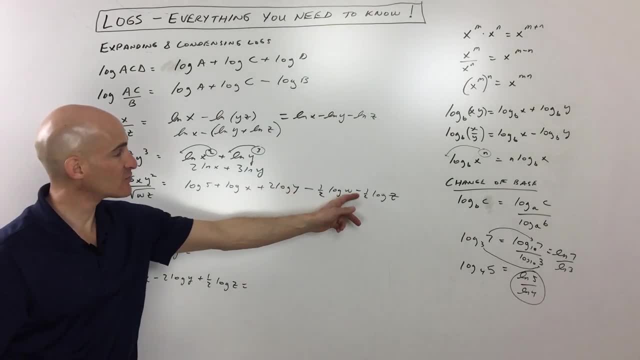 I just wanted to show you a more challenging one. but notice, everything that's in the denominator is being subtracted. The square root is the one half power, so I brought that one half down in front. Same thing with here the Y squared. 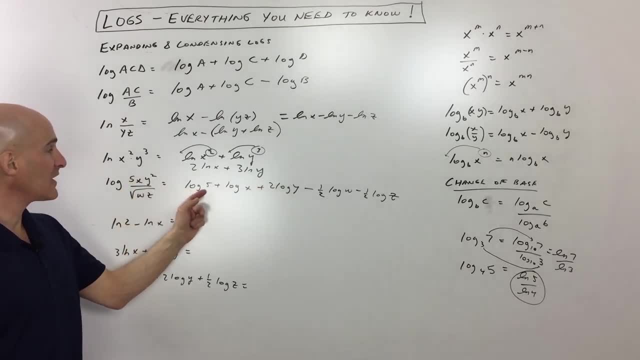 I brought that two down in front. Everything that was in the numerator that was multiplied together. I wrote it as a sum of logs, and the ones that were in the denominator I subtracted. Okay, that's the quotient rule. Now we're gonna go over to the condensing. 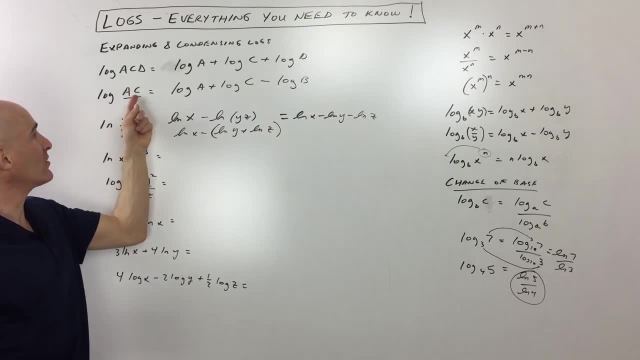 denominator. you're going to be subtracting. whatever's in the numerator is going to be positive, you're going to be adding okay. so that's just a quick way to figure these ones out, but you can do it in steps like this too: this one: we've got some exponents here, so this is actually going. 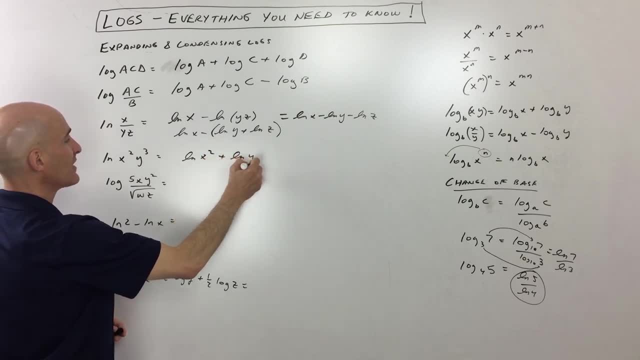 to be natural log of X squared plus natural log of Y cubed, because you can see these are multiplied. so I wrote it as a sum of two logs. then what I'm going to do is I'm going to bring those powers down in front as coefficients. that's the power property. okay for log. so this is going to be two. 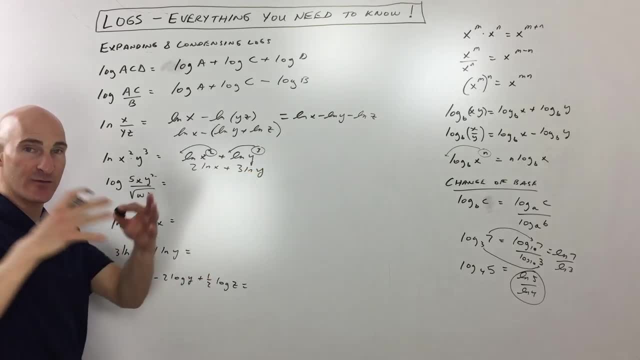 natural log of X plus three natural log of Y, that's fully expanded. and then one here this is pretty more challenging- one, let's see it's log of. let's see log of five plus log of X plus two log of Y. see, I brought down that two in front, okay, and then minus, because we're dividing one half. 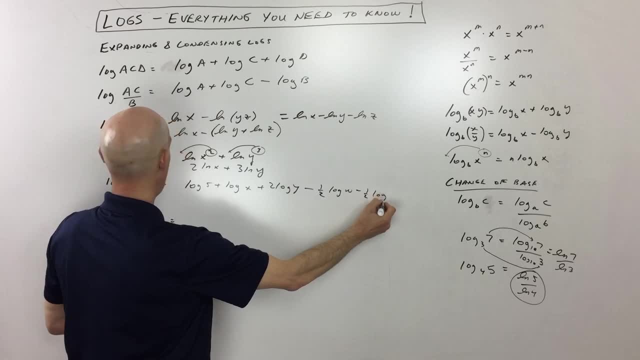 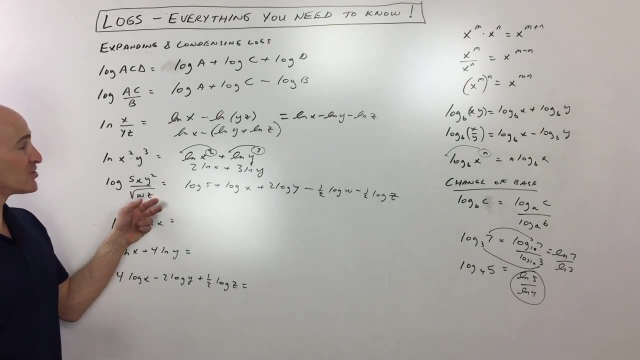 log of W minus one half log of Z. so I did all that in one step. now you don't have to do it in one step like I did. I just want to show you a more challenging one. but notice, everything that's in the denominator is being subtracted. the square root is the one half power, so I brought that one. 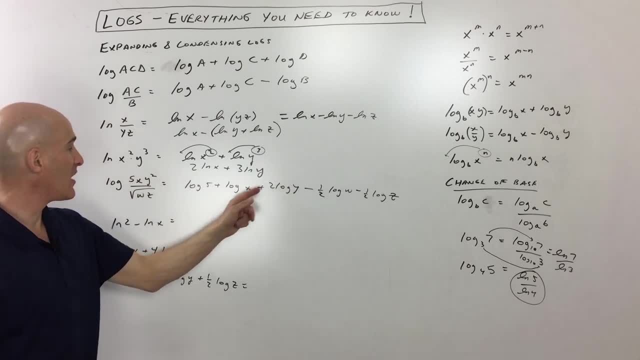 half down in front. same thing with here the Y squared. I brought that two down in front. everything that was in the numerator that was multiplied together. I wrote it as a sum of logs and the ones are in the denominator I subtracted. okay, that's the quotient rule. now we're going to go. 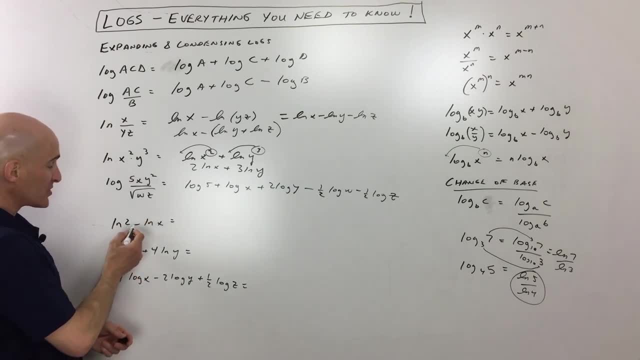 over to the condensing. so we want to condense these into one log. so we're subtracting. so what I'm going to do is I'm going to divide, and don't get confused. you want to make sure the one that comes first or to the left is. 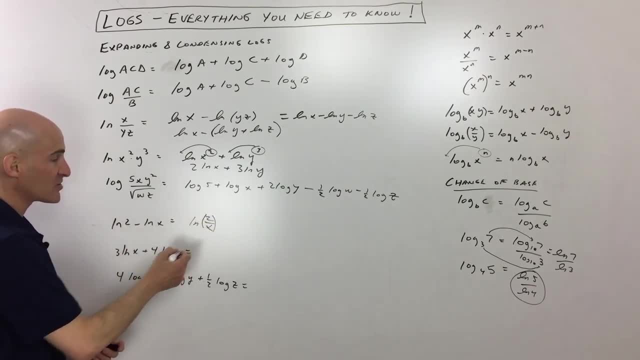 in the numerator, the one you're subtracting, that one goes in the denominator. so it's like natural log of two divided by X, this one with the coefficients. I would bring those up as powers first and then you can put it all together. so this would be natural log of X cubed times Y to. 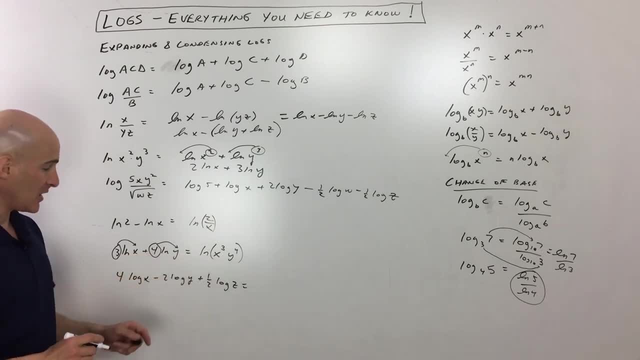 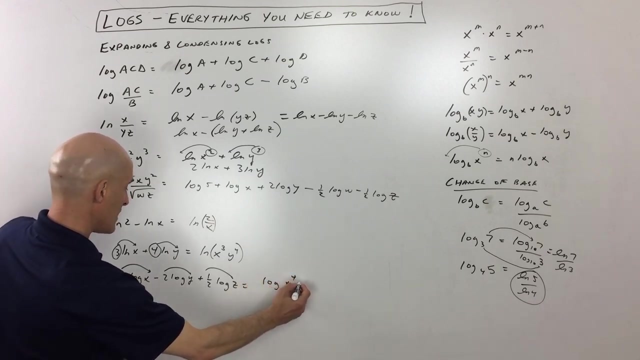 the fourth: okay, adding. so we multiplied. okay, and then this last one. we've got quite a bit going on here, so I'm going to bring up the coefficients. okay, one half is going to make that the square root of Z. so if I do, this is going to be log of X to the fourth, right over. 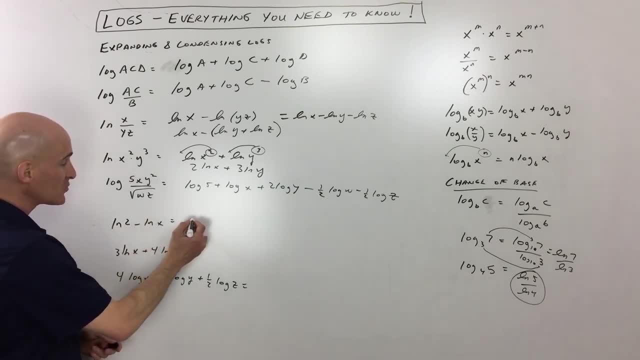 So we wanna condense these into one log. So we're subtracting. so what I'm gonna do is I'm gonna divide and don't get confused. You wanna make sure the one that comes first or to the left is in the numerator. 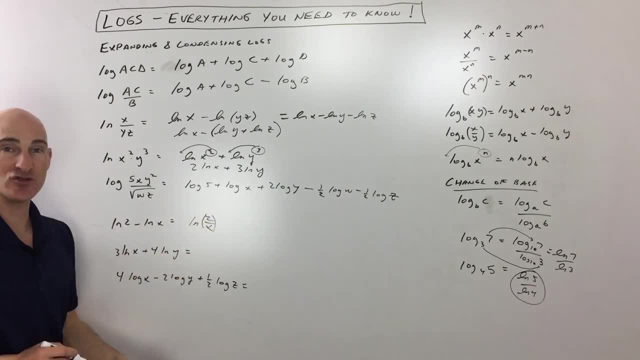 The one you're subtracting. that one goes in the denominator. So it's like natural log of two divided by X, This one with the coefficients. I would bring those up as powers first, and then you can put it all together. 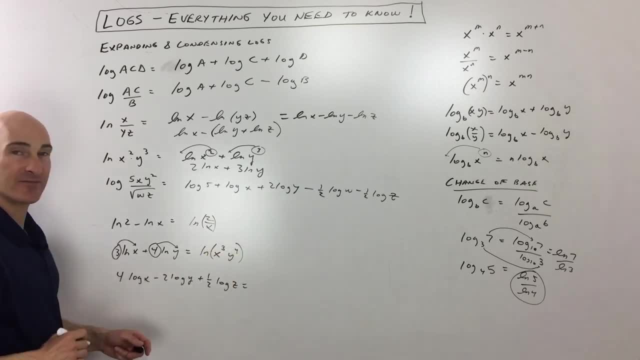 So this would be natural log of X cubed times Y to the fourth, okay Adding, so we multiplied, okay, And then this last one. we've got quite a bit going on here, so I'm gonna bring up the coefficients, okay. 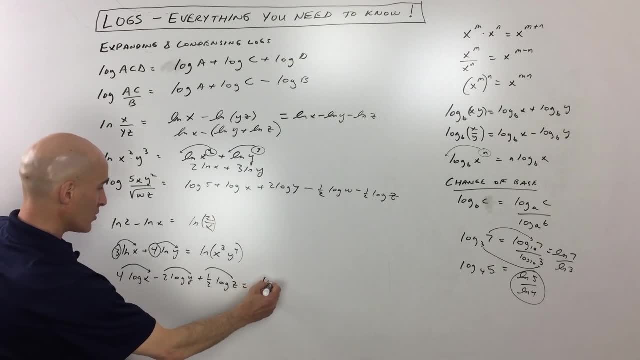 One half is gonna make that the square root of Z. so if I do this it's gonna be log of X to the fourth right over. see, because we're subtracting Y squared plus, that's gonna be times the square root of Z. 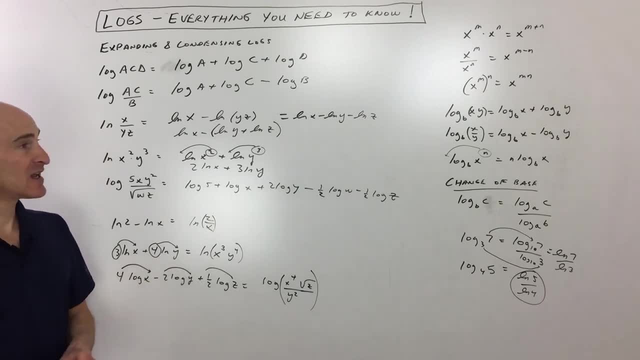 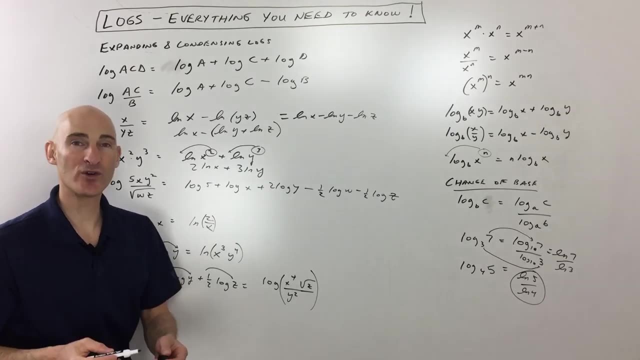 So that was a more challenging one. So this has been expanding and condensing logs. Now we're gonna get into evaluating equations and solving equations using logarithms, So let me erase this board and we'll get back with that. Okay, now we're gonna solve equations using logarithms. 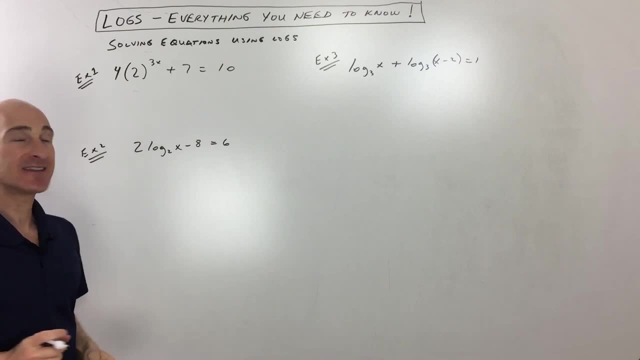 So, just like algebra, you wanna work from the outside in, You wanna try to isolate that variable. Same thing here. we're trying to get that X by itself. So let's go ahead and subtract seven from both sides, So that gives us four times two. 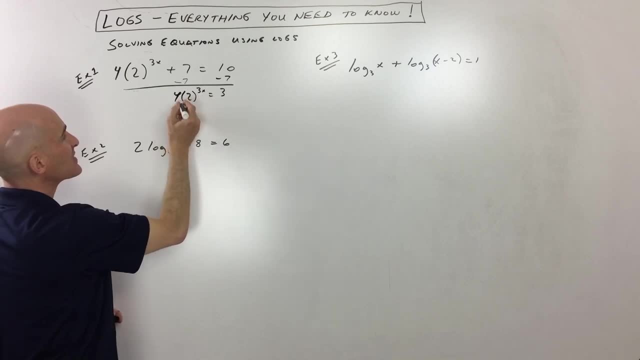 to the three, X, power equals three. Again, working from the outside in, let's divide both sides by four. So now we have two to the three, X equals three, fourths, Whenever that variable's in the exponent position. okay, you need to get it down from there. 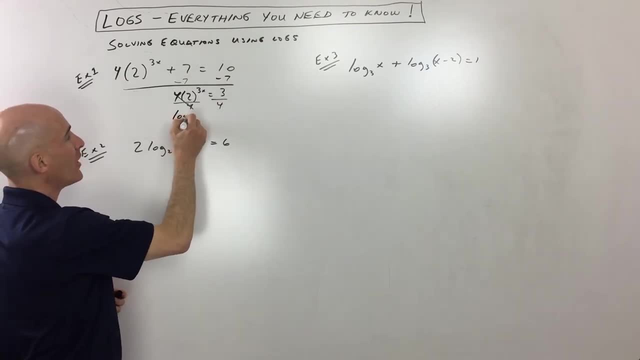 We need to reverse that exponentiation process. We wanna take the log base two, okay, of both sides of the equation to keep it balanced right. So the log base two and the exponential base two, those cancel. So now we have three X equals log base two of three fourths. 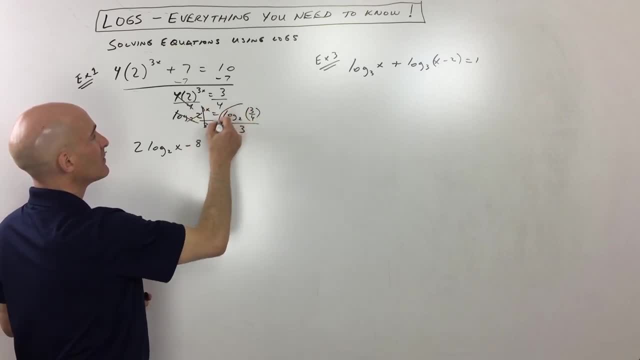 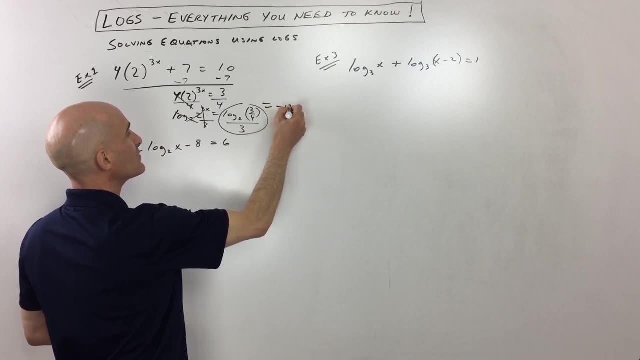 If we divide both sides by three, that's it. you got it. Now you can do that in your calculator. I did that here. for us It's a negative .138 approximately. Okay, let's go to example number two. Same thing here. you're trying to work from the outside in. 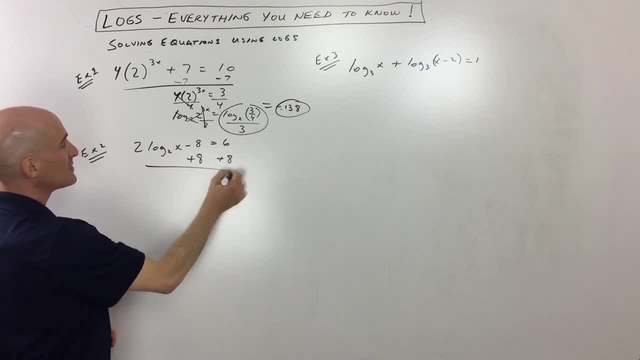 You're trying to get that X by itself. So let's add eight to both sides, So that gives us two log base two of X equals 14.. Let's divide both sides by two. We're still working from the outside in. We've got log base. two of X equals seven. 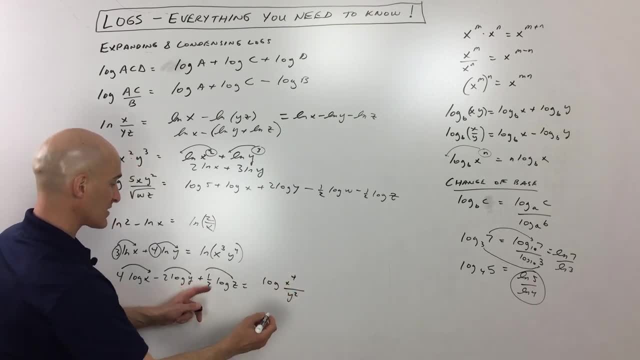 because we're subtracting Y squared plus that's going to be times the square root of Z, so that was a more challenging one. so this has been expanding and condensing logs. now we're going to get into evaluating equations and solving equations using logarithms. So let me erase. 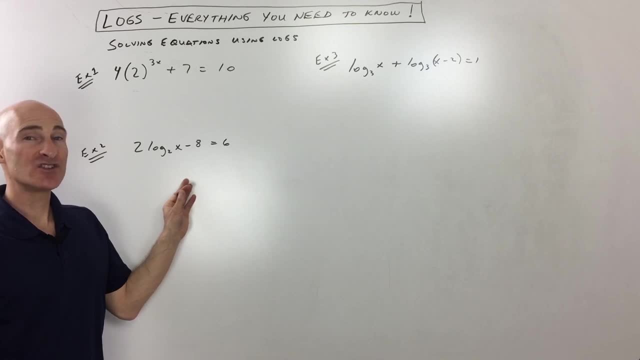 this board and we'll get back with that. Okay, now we're going to solve equations using logarithms. So, just like algebra, you want to work from the outside in, You want to try to isolate that variable. Same thing here: We're trying to get that x by itself. So let's go ahead and subtract. 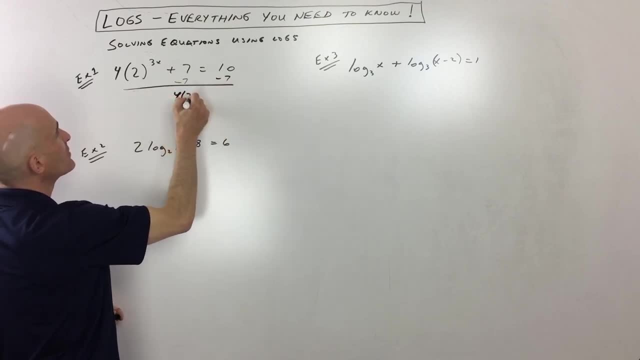 7 from both sides. So that gives us 4 times 2 to the 3x power equals 3.. Again, working from the outside in, let's divide both sides by 4. So now we have 2 to the 3x equals 3 fourths. Whenever. 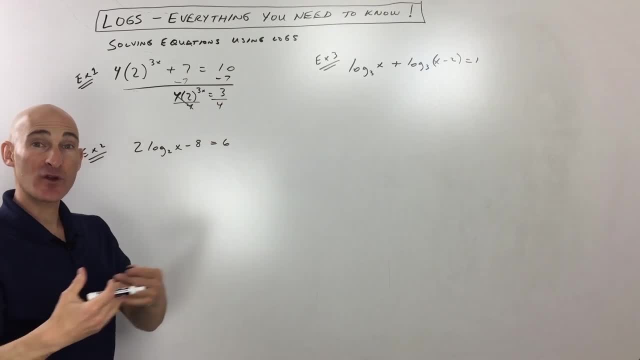 that variable is in the exponent position. okay, you need to get it down from there. We need to reverse that exponentiation process. We want to take the log base 2, okay- of both sides of the equation to keep it balanced, right. So the log base 2 and the exponential base 2, those cancel. 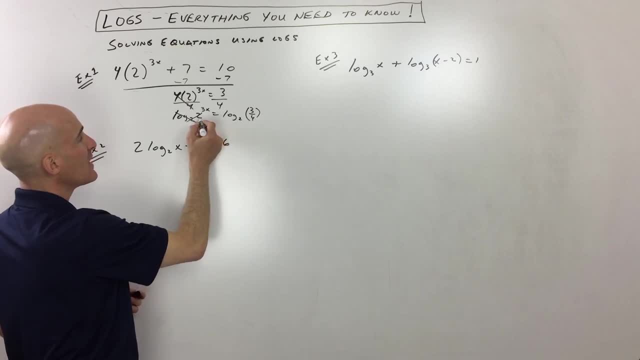 So now we have 3x equals log base 2 of 3 fourths If we divide both sides by 3, okay, that's it. You got it. Now you can do that in your calculator. I did that here for us, It's. 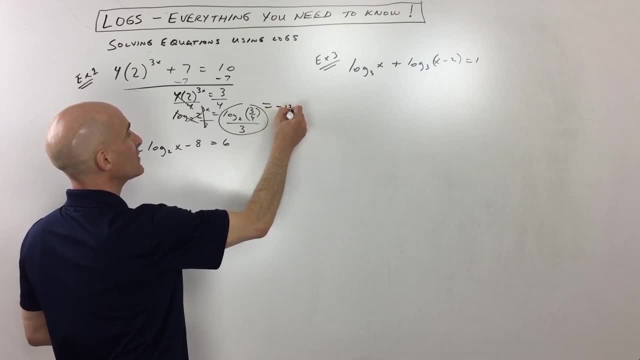 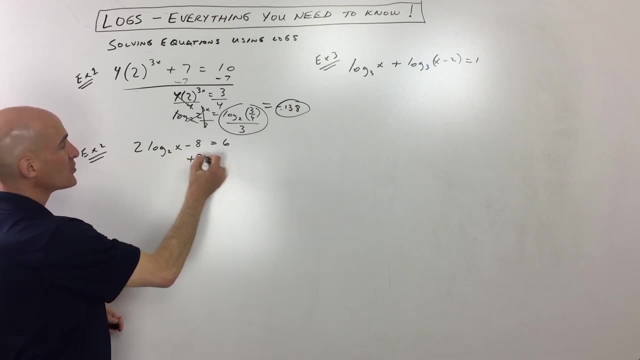 negative: 0.138 approximately. Okay, let's go to example number 2.. Same thing here. You're trying to work from the outside in. You're trying to get that x by itself. So let's add 8 to both sides, So that gives us 2 log base 2 of x equals 14.. Let's divide both sides by 2.. We're still. 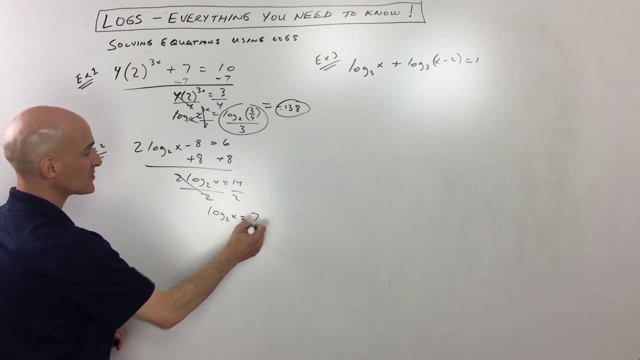 working from the outside in. We've got log base 2 of x equals 7. We want to get that variable by itself. What's the inverse of taking the log base 2?? Well, we're there, So we're going to do x plus 2.. Let's put 2 minus 2x. We can do x plus. 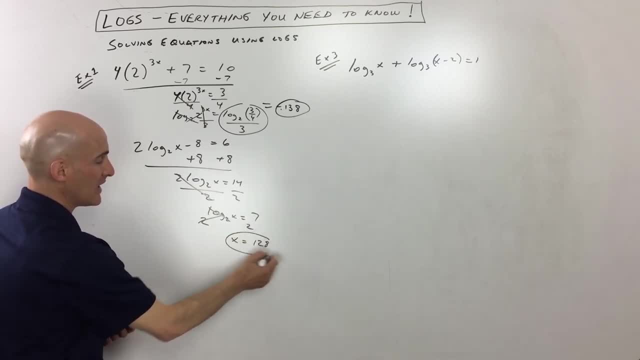 2.. Let's do 2 minus 2x, So that gives us x plus 2.. So we have: x equals 2 to the 7th power, which is 128.. Okay, in example number 3, here we're going to use the properties of logs to. 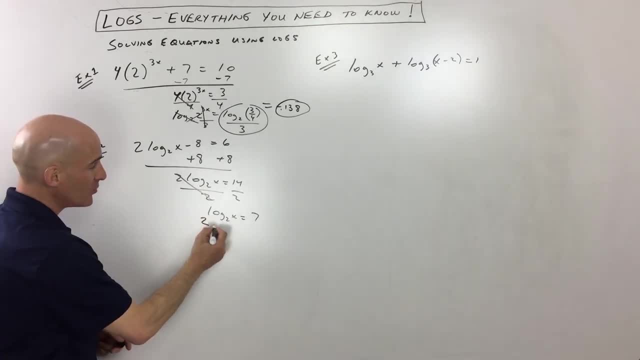 We wanna get that variable by itself. What's the inverse of taking the log base two, exponentiating using base two? So we have: X equals two to the seventh power, which is 128.. Okay, in example number three, here we're gonna use the properties of logs. 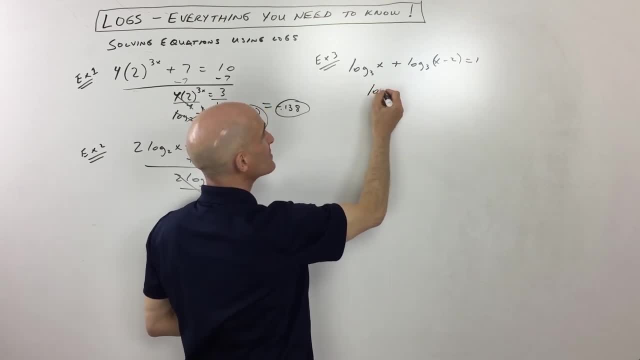 to condense these into one log. Remember, when you're adding, what do you do to the arguments? You multiply them, So that's gonna be X squared minus two X. I'm multiplying those together equals one. And then again we're trying to work from the outside in. 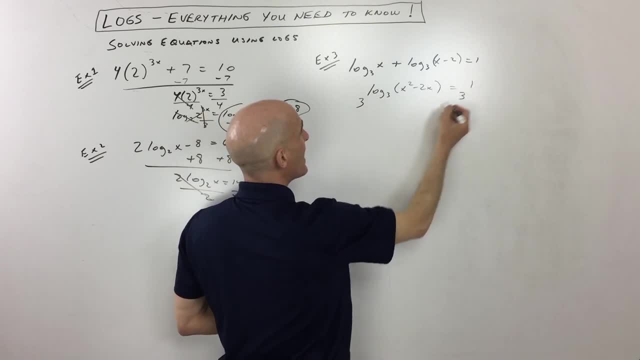 We're trying to get that variable by itself. So let's exponentiate both sides. So I'm raising base three. So those cancel one another out. We get X squared minus two. X equals three. I'm gonna subtract three from both sides. 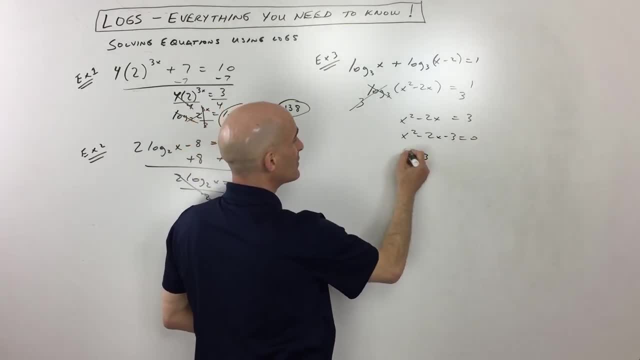 Set this equation equal to zero. I'm gonna factor- It's all coming back to you from earlier in math, right, And then now, if we set these factors to zero, we get X equals three or negative one. But the one thing you wanna be careful with, 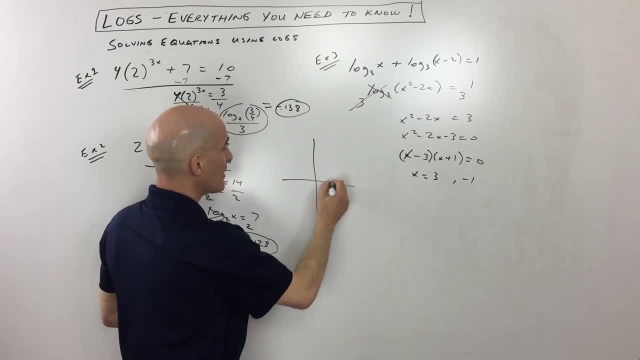 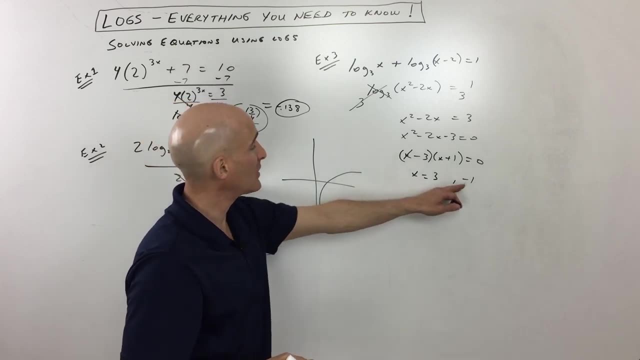 with log equations because, remember, the graph looks like this: right Log. you can't take the log of zero. You can't take the log of a negative number. That's not in the domain, okay. So if we look at negative one, 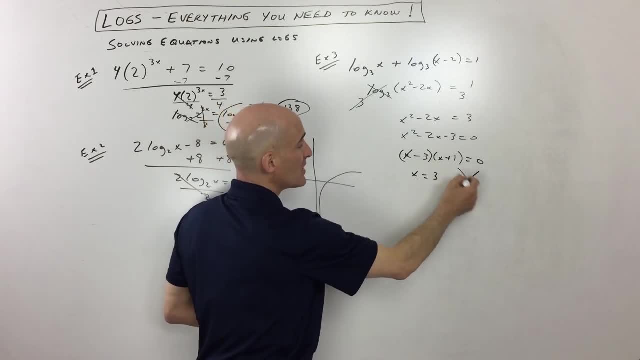 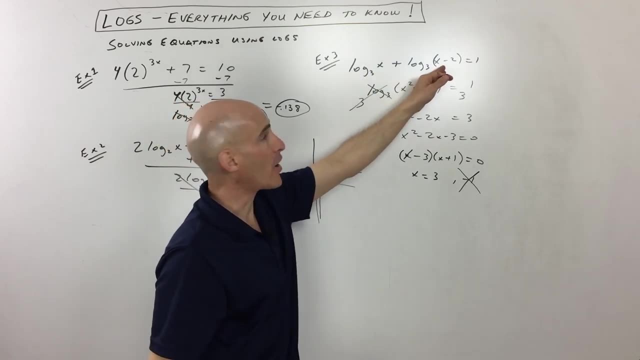 so you'd be taking the log of a negative one. a negative number, that's extraneous, That's not possible. Three's: okay, We're not gonna be taking the log of zero or negative value, But when you simplify that argument, okay. 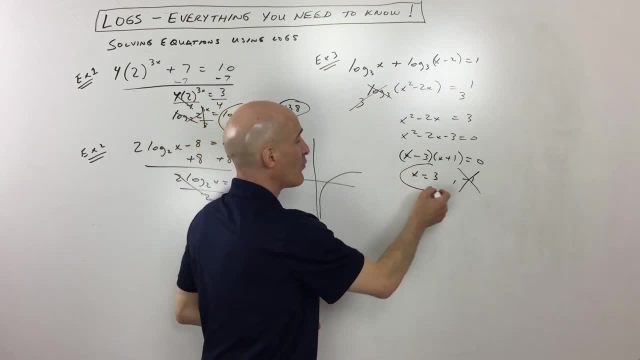 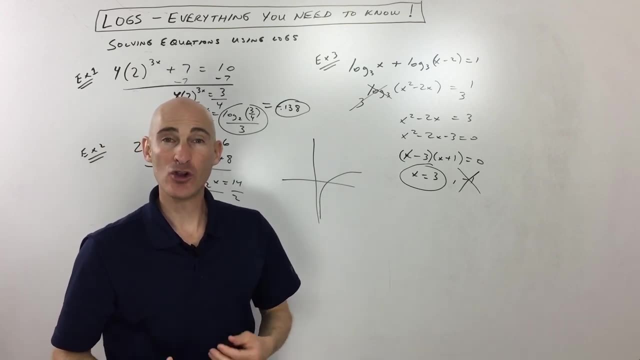 So that has to be a positive value. once you simplify So it looks like we just have one answer: X equals three and you got it. So we did quite a bit here in this video giving you all you need to know about logs. 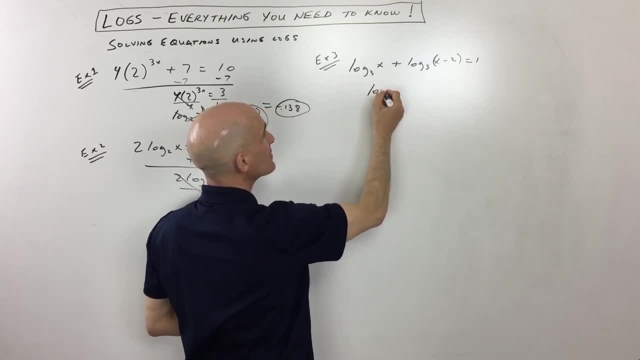 condense these into one log. Remember, when you're adding, what do you do to the arguments? You multiply them, So that's going to be x squared minus 2x. I'm multiplying those together equals 1.. And then again we're trying to work from the outside in, We're trying to get that variable by. itself. So let's exponentiate both sides of the equation, Then we'll move it to one. So we have log base 2 of x equals 14.. We're trying to get that variable by itself. So let's exponentiate both sides by. 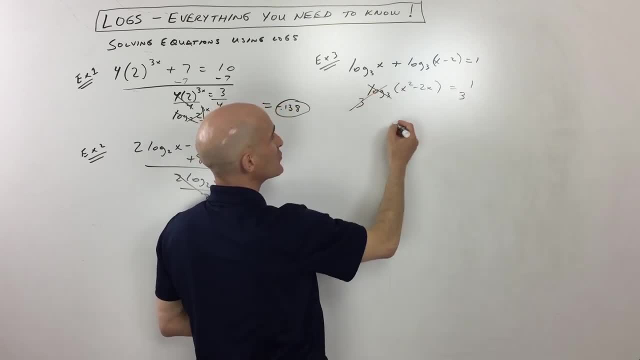 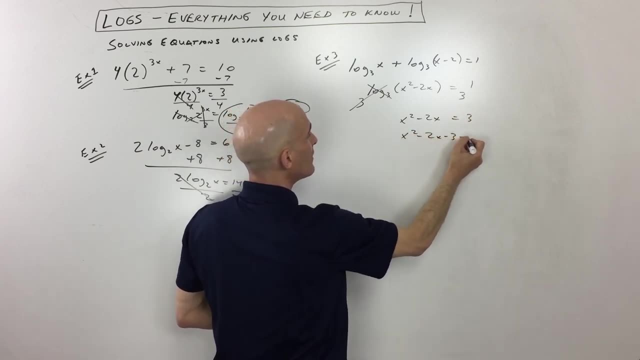 exponentiate both sides. so i'm raising base three. so those cancel one another out. we get x squared minus 2x equals 3. i'm going to subtract 3 from both sides. set this equation equal to zero, i'm going to factor. okay, so this is all coming back to you from earlier in math, right, and then now. 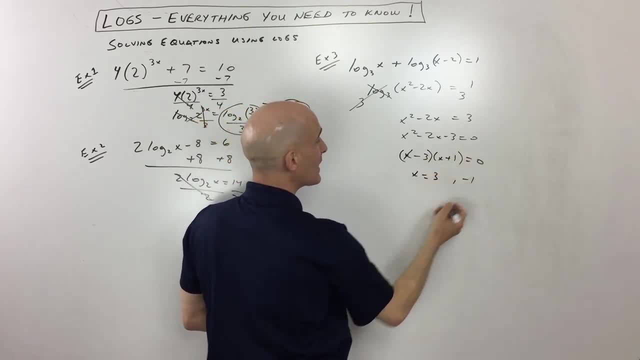 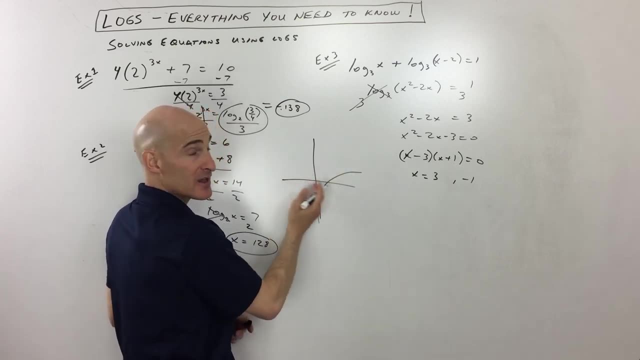 if we set these factors to zero, we get x equals 3 or negative 1. but the one thing you want to be careful with with log equations because, remember, the graph looks like this: right log: you can't take the log of zero, you can't take the log of a negative number. that's not in the domain, okay, so 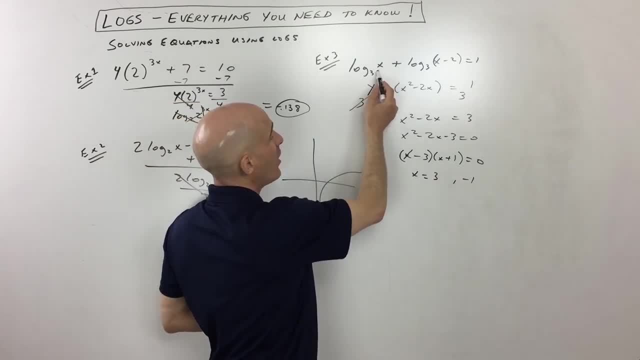 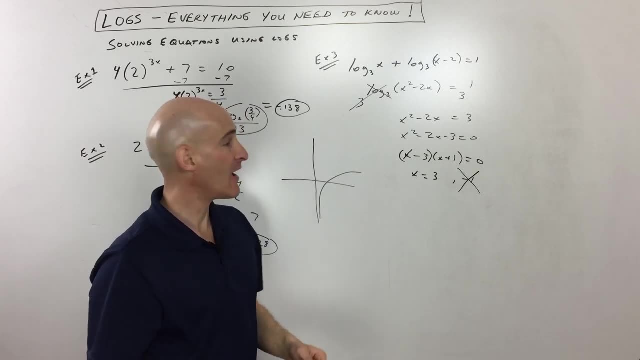 if we look at negative one, so you'd be taking the log of a negative one, a negative number. that's extraneous, that's not possible. three is okay. we're not going to be taking the log of zero or a negative value when you simplify that argument. okay, so that has to be a positive. 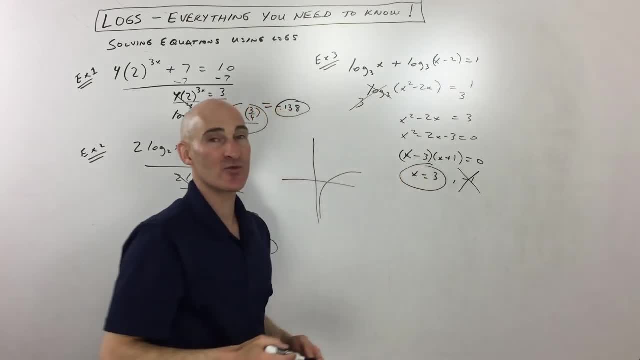 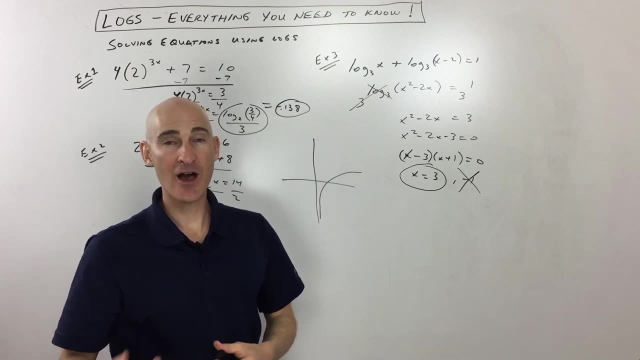 value once you simplify so it looks like we just have one answer: x equals three and you got it. so we did quite a bit here in this video, giving you all you need to know about logs, from evaluating you to solving equations, to expanding, condensing, graphing. i hope you like this video. subscribe. 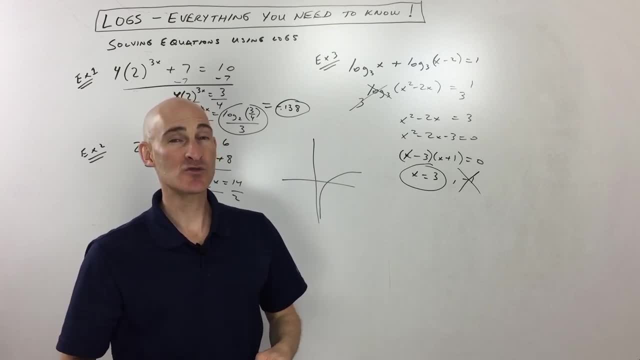 to the channel. check out more math tutoring videos on my youtube channel, mario's math tutoring. and i want to mention, if you're preparing for the act or the sat, check out my huge act math review video course or my huge sat math review video course, packed with tons of information. if 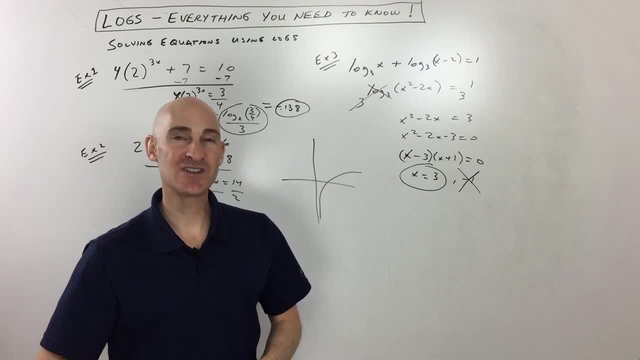 you like my teaching style. you'll get a lot of those courses and i look forward to seeing you in the future videos. i'll talk to you soon. 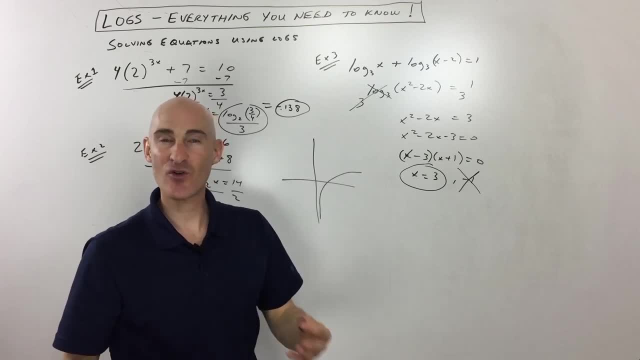 from evaluating to solving equations, to expanding condensing graphing. I hope you liked this video. Subscribe to the channel. Check out more math tutoring videos on my YouTube channel, Mario's Math Tutoring. And I wanna mention, if you're preparing for the ACT, 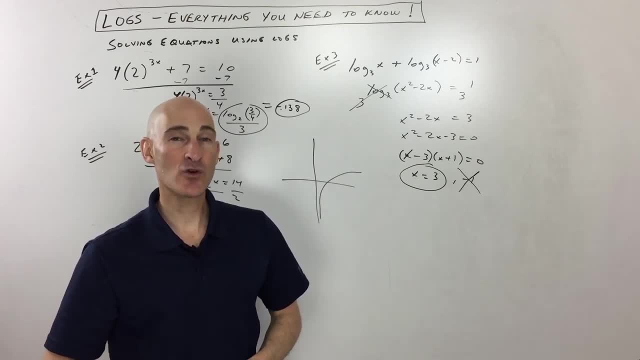 or the SAT. check out my huge ACT math review video course Or my huge SAT math review video course, packed with tons of information. If you like my teaching style, you'll get a lot of those courses And I look forward to seeing you in the future videos. I'll talk to you soon.